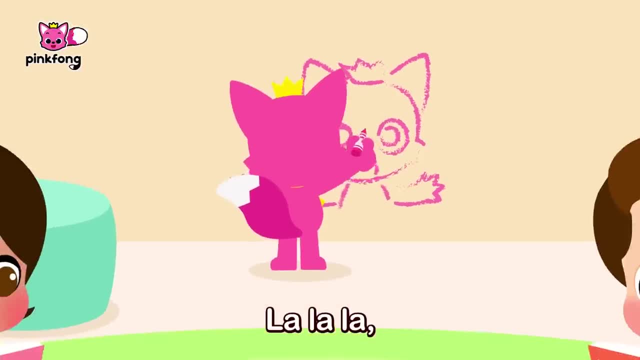 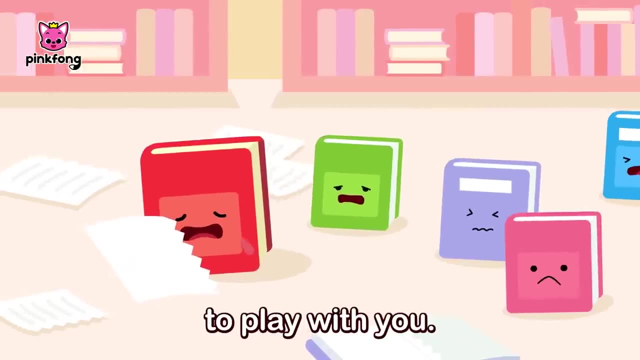 Draw the wall. doodle doodle. it is so much fun. La, la, la, la, la la la. doodle doodle. It hurts so much, very much. I don't want to play with you anymore. 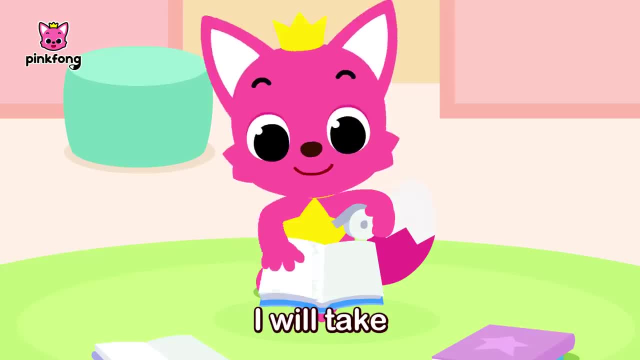 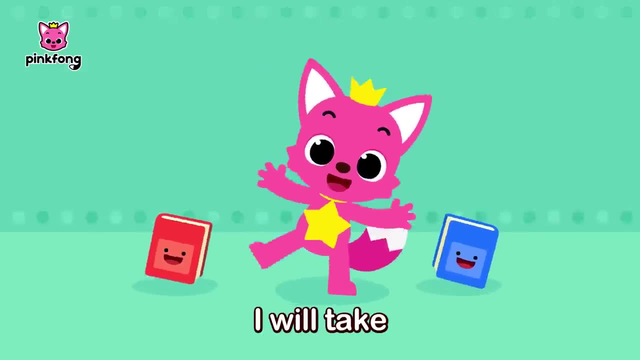 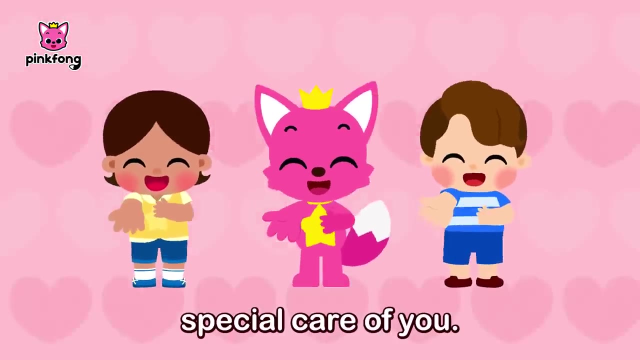 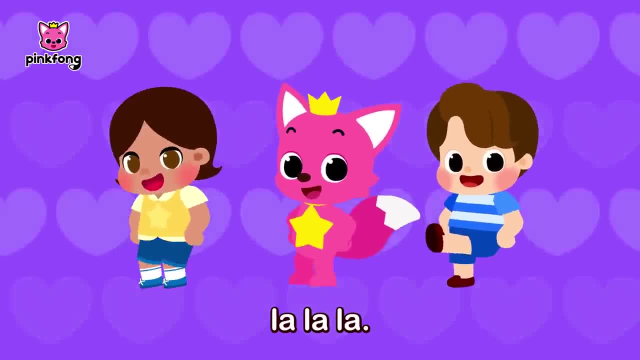 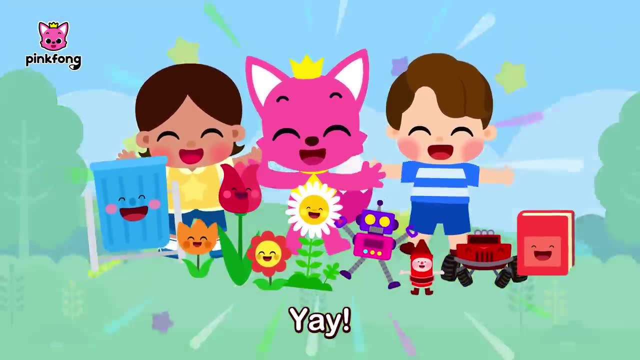 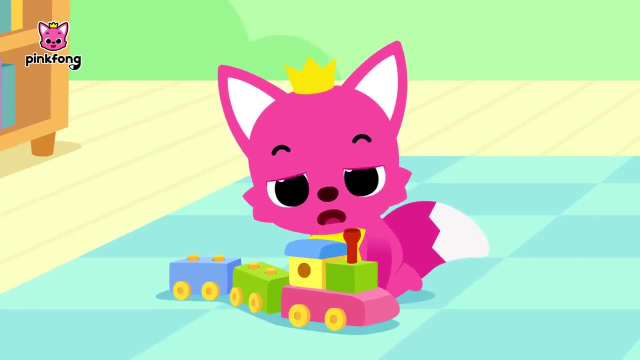 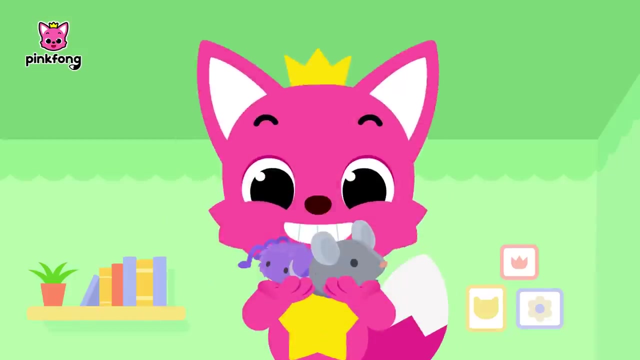 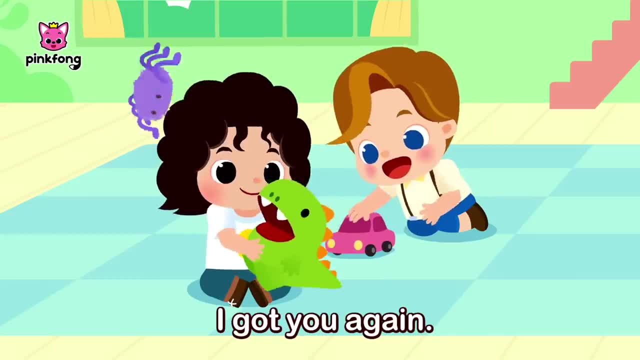 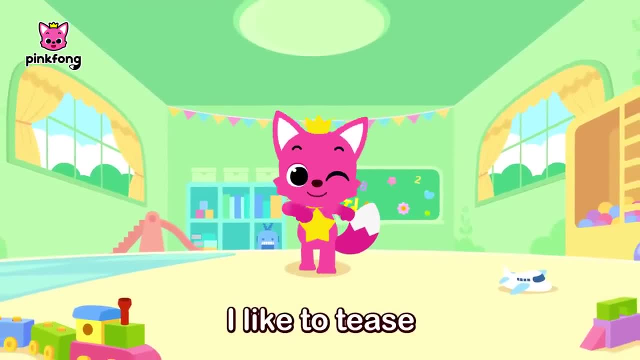 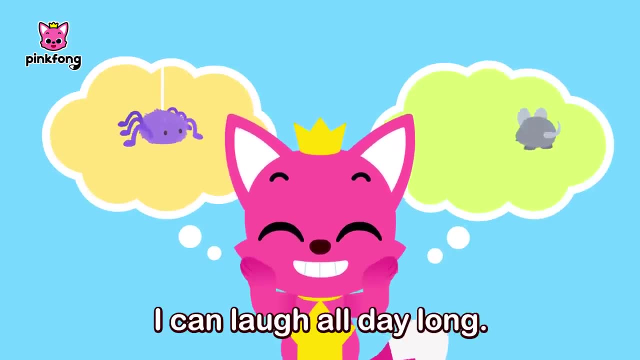 Stop it, Minfrog. Hello, I like to tease my friends all day long. Teasing, teasing. It's so much fun. I can laugh all day long. There's a big spider, there's a big mouse, Watch out, everyone, run, run, run. 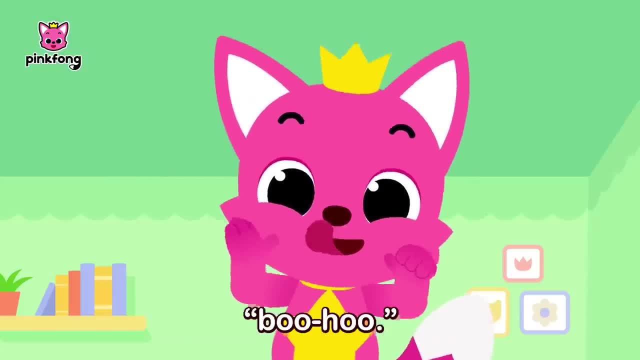 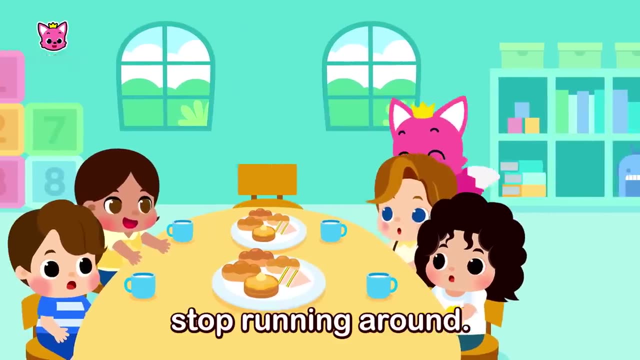 Here I go boo, there I go boo. It's so fun making them boo-hoo. Okay, everyone take a seat now. Pinkfong, stop running around. Oh no, you spilled my milk. I didn't do it. no, not me. 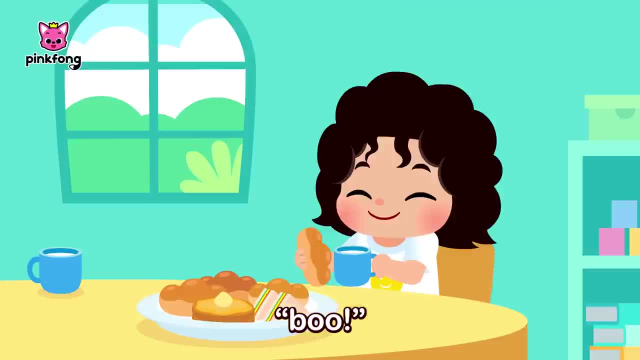 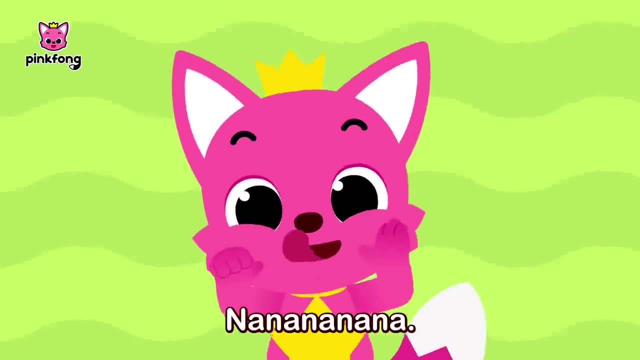 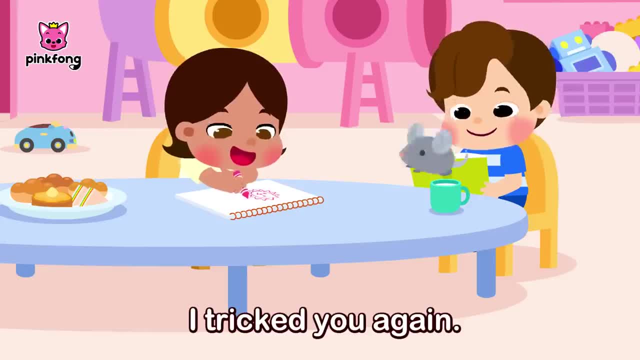 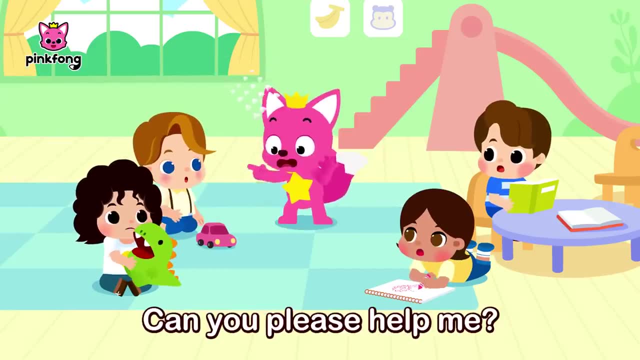 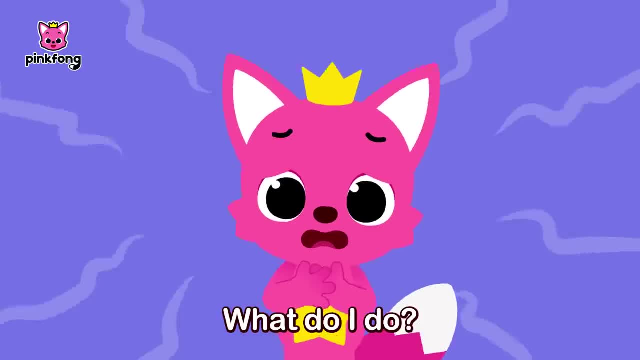 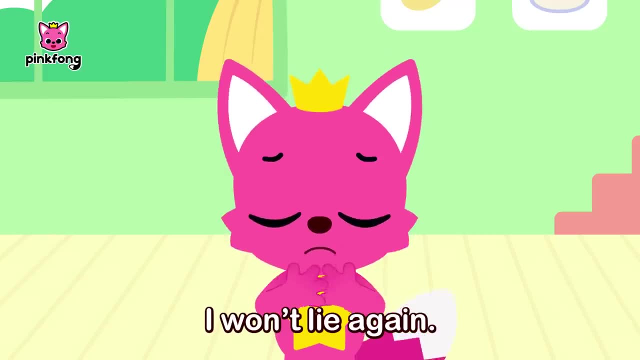 This time we won't be tricked by you. What do I do? No one trusts me. What, what, what, What do I do, do, do. What do I do? No one helps me. I won't lie again. 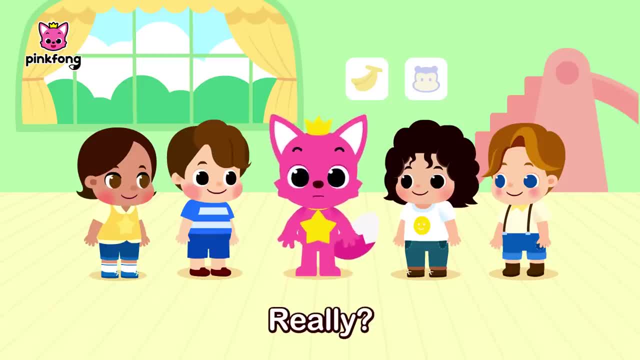 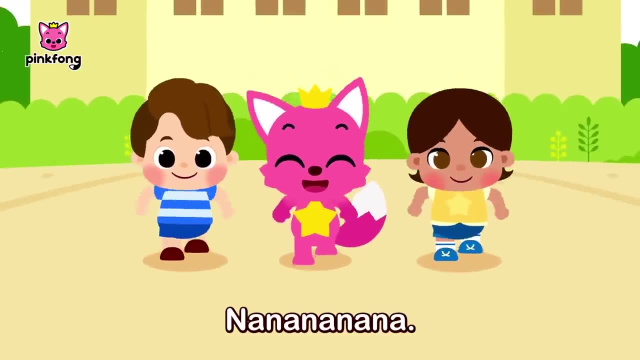 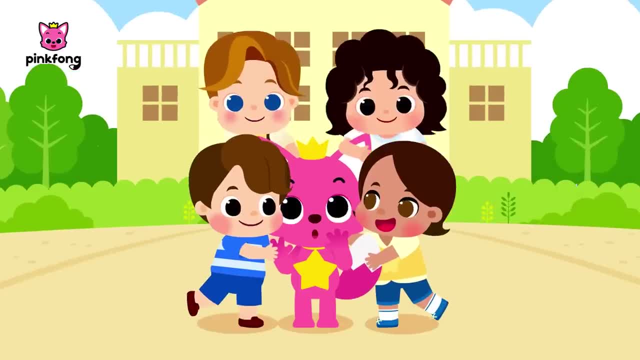 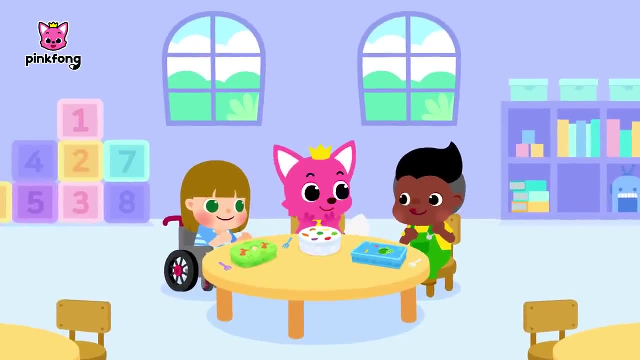 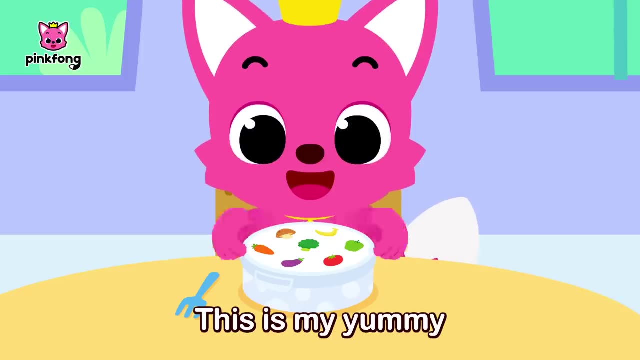 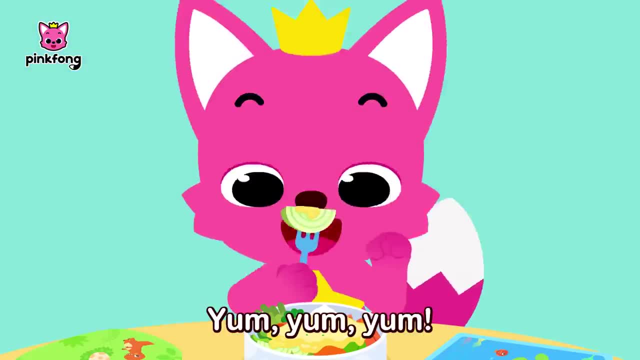 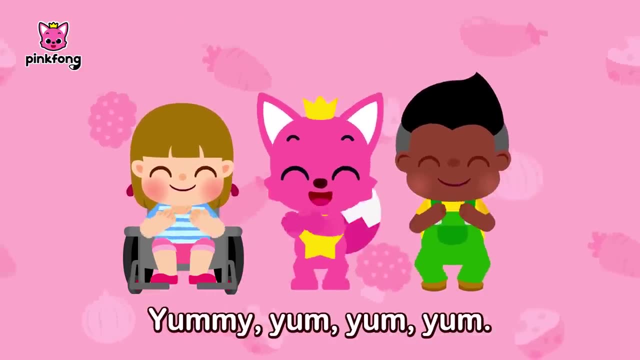 On top, All so healthy and looks yummy yum, yum, yum. We love your lunchbox, Lunchbox. Yummy yum yum. Yummy, yum, yum, yum. Let's try this and that different taste: Yummy, yum yum. 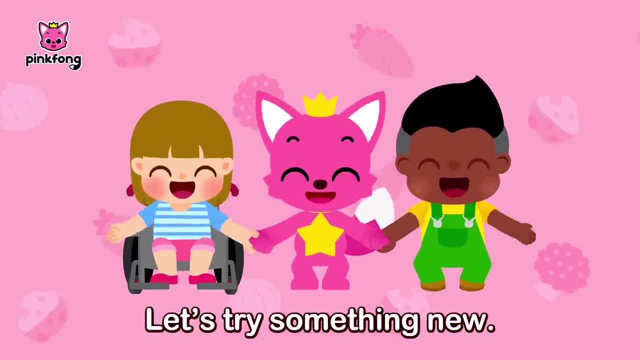 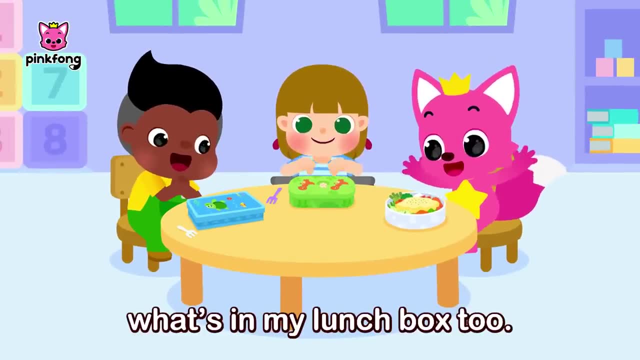 Yummy, yum, yum, yum. Let's try something new. Yum, yum, Wow. your lunchbox looks so yummy. I'll show you what's in my lunchbox too. This is my yummy meat lunchbox: Roasted chicken with potatoes on the side. 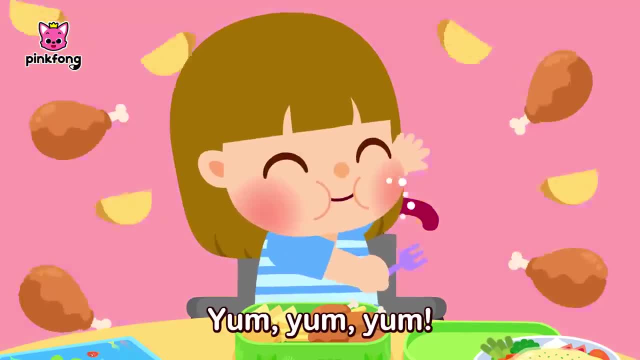 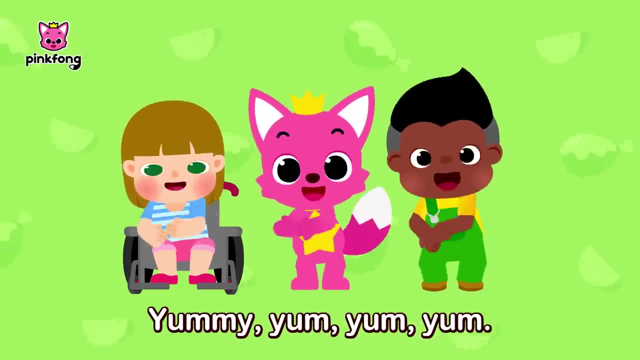 On the side, All so healthy and looks yummy yum, yum yum. We love your lunchbox, Lunchbox. Yummy yum yum. Yummy yum, yum, yum. Let's try this and that different taste: Yummy yum yum. 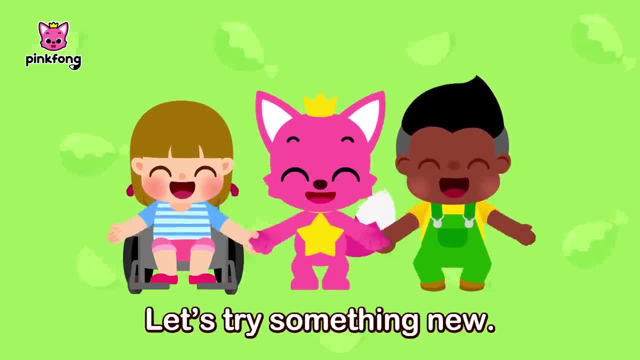 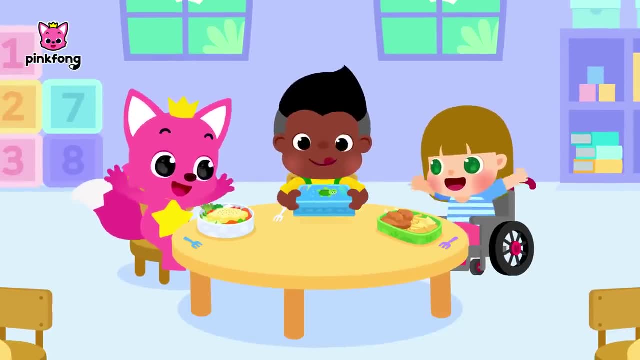 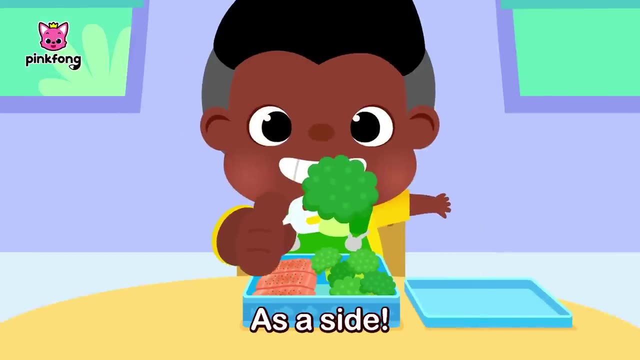 Yummy, yum, yum, yum. Let's try something new. Yum, yum, Cool. Can you guess what's in my healthy lunchbox? This is my yummy seafood lunchbox: Seasoned salmon with broccoli as a side. As a side, All so healthy and looks yummy, yum, yum yum. 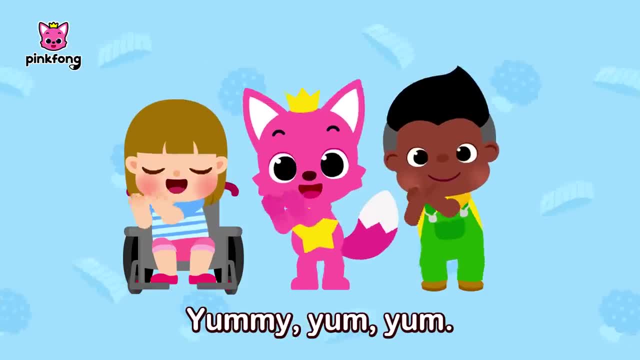 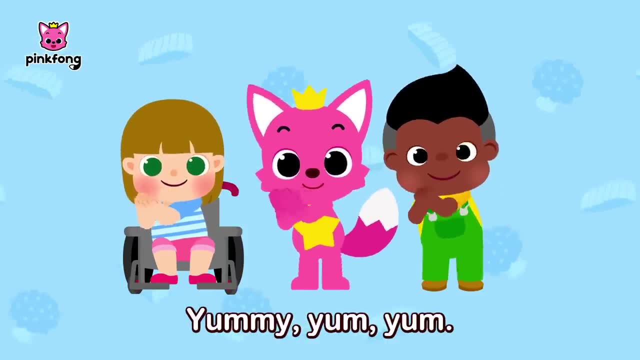 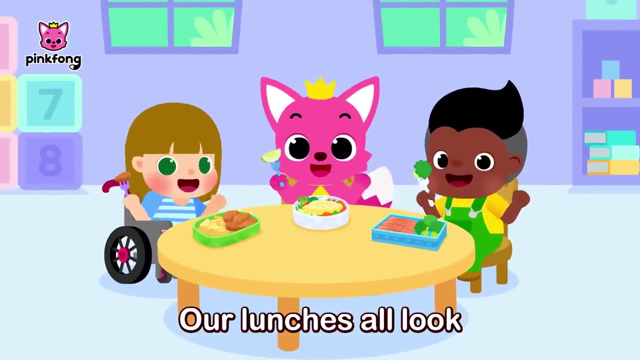 We love your lunchbox, Lunchbox. Yummy, yum, yum, Yummy, yum, yum, yum. Let's try this and that different taste. Yummy yum, yum, Yummy, yum, yum, yum. Let's try this and that different taste. 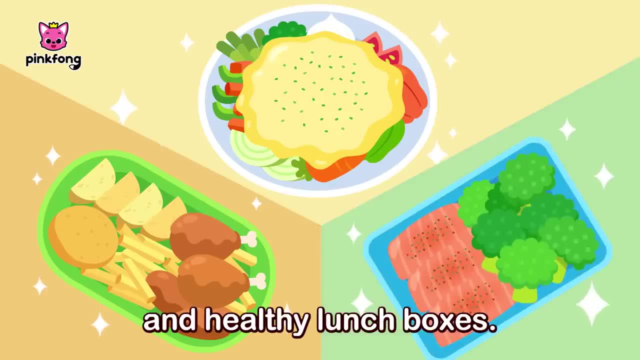 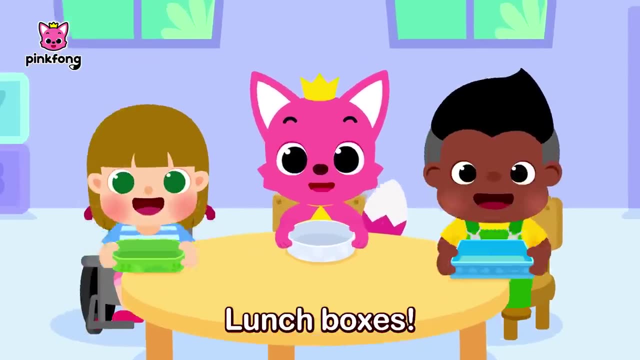 Yummy, yum, yum, Yummy, yum, yum, yum. Let's try something new. Yum yum, Our lunches all look so delicious. Yeah, Our yummy special lunchboxes. All so colorful and healthy lunchboxes. Yum yum, yummy, yum, yum yum. Let's try this in a different taste. 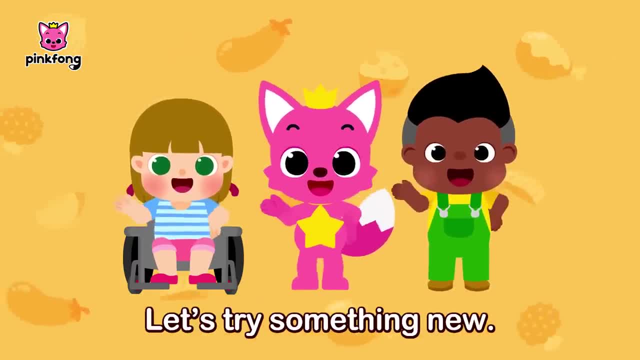 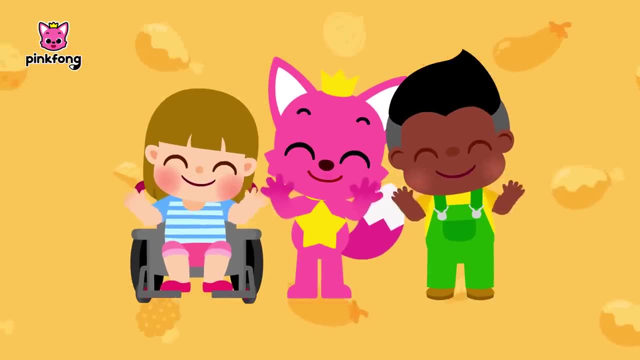 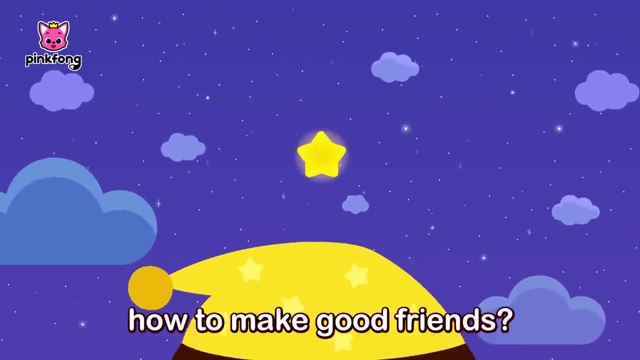 Yummy, yum, yum, yummy, yum, yum, yum. Let's try something new. Yum yum, all healthy and delicious. Tomorrow is my first day of school. Starlight, can you tell me how to make good friends? 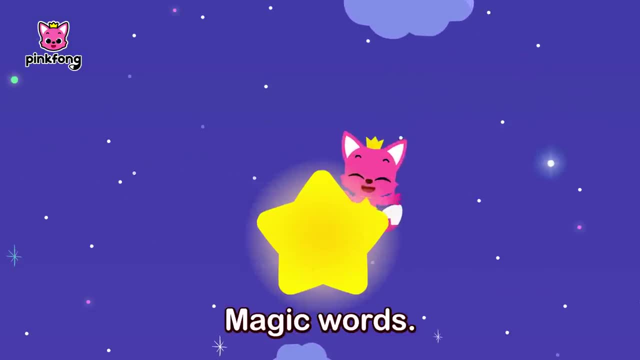 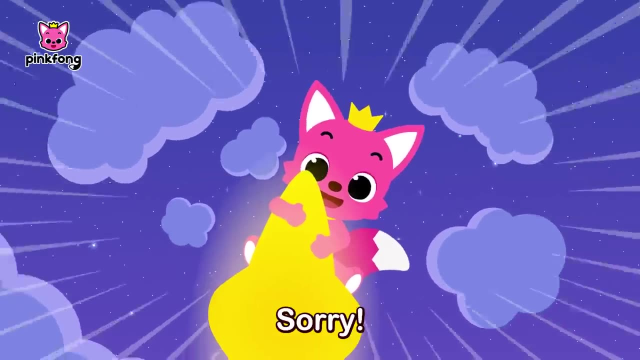 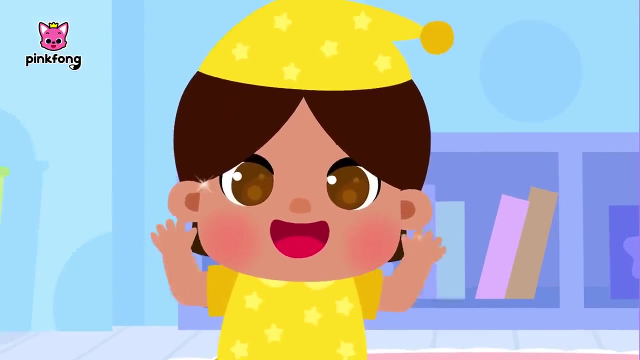 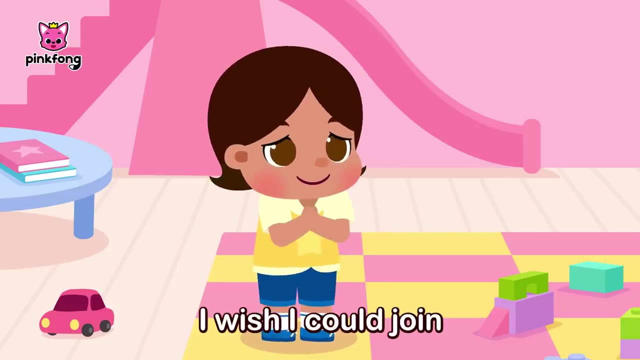 Magic words, magic words for you and me. Magic words, magic words. remember these magic words. Blocks, blocks, well colorful block, a soul. I wish I could join those kids. Oh, what, what, what, what should I say to those kids? 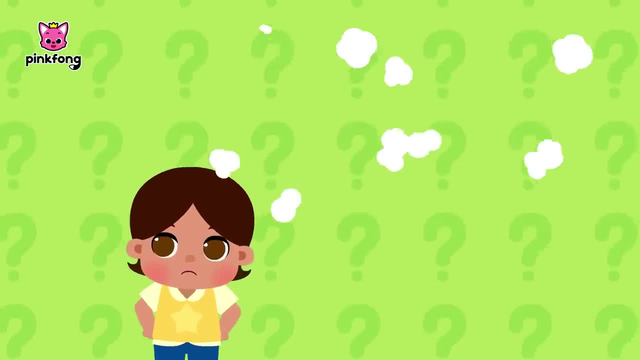 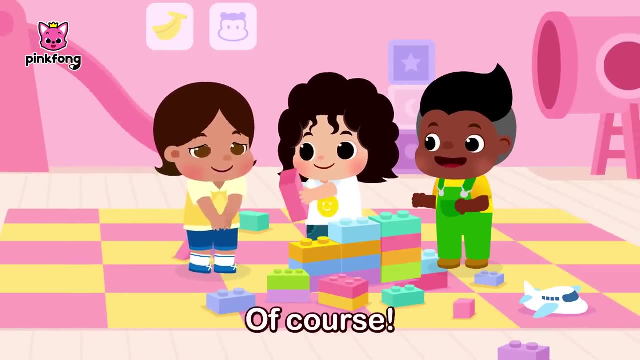 Remember those kids, Remember those kids, Remember the magic words: A hug, please, and thank you. Can I join you please? Can I join you please? Yes, yes, of course, Yes, of course, Oh, yay, Thank you. thank you, my friends. 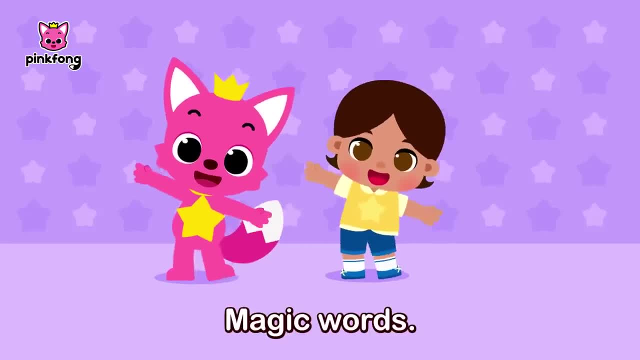 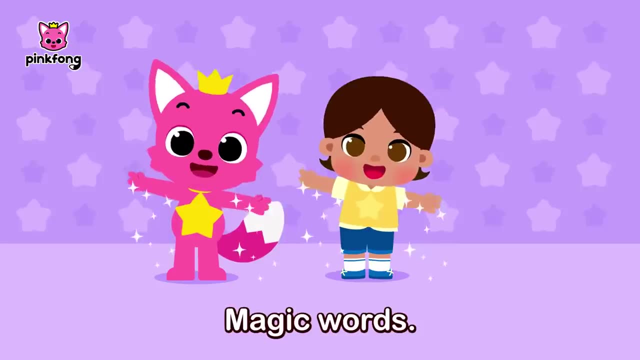 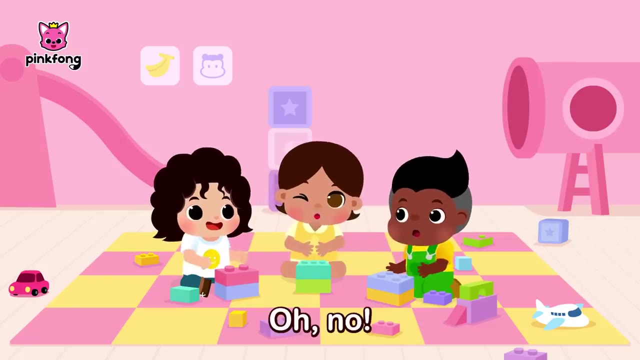 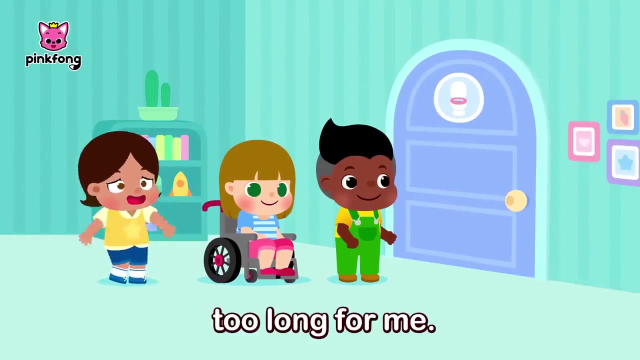 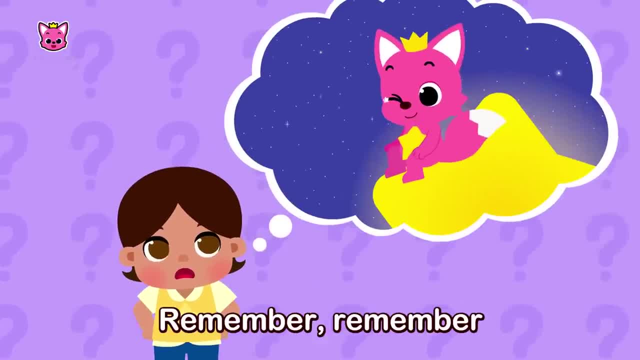 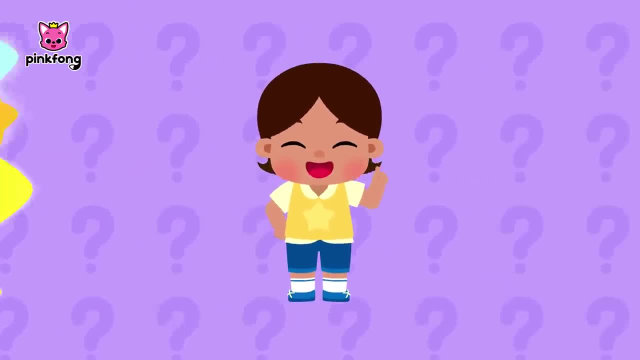 Now, what, What, What? What should I say to my friends? Remember, remember the magic words: Uh-huh, Excuse me and sorry, Excuse me, my friends, Excuse me, my friends. I'm sorry, but can I go. 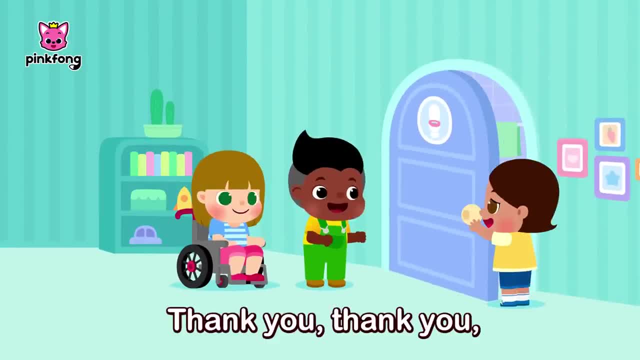 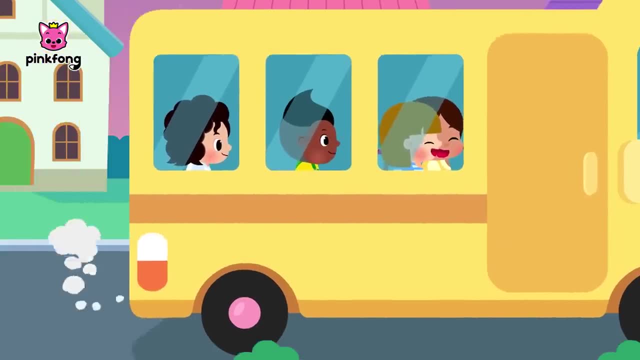 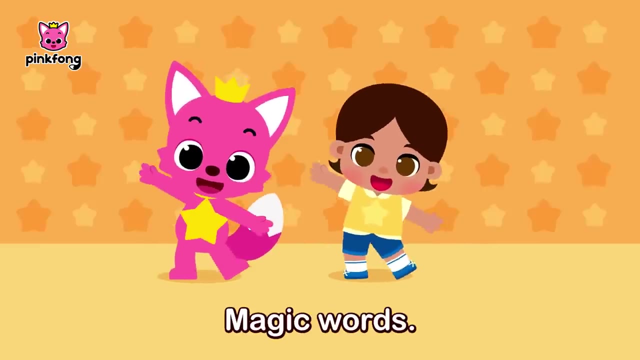 First, please, sorry, Of course, Thank you. thank you, my friends, Always. always. here's your magic words. Magic words, please. Magic words, thank you. Magic words for you and me. Magic words, excuse me, Magic words, sorry. Remember these magic words. 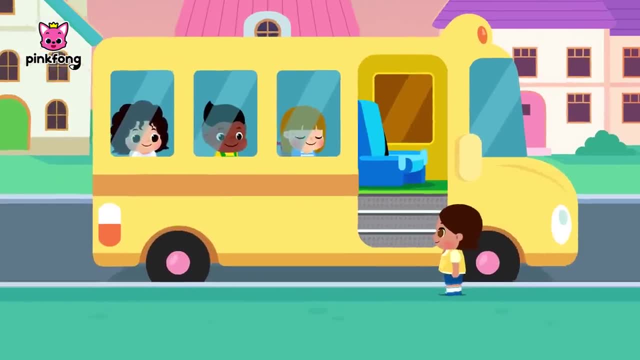 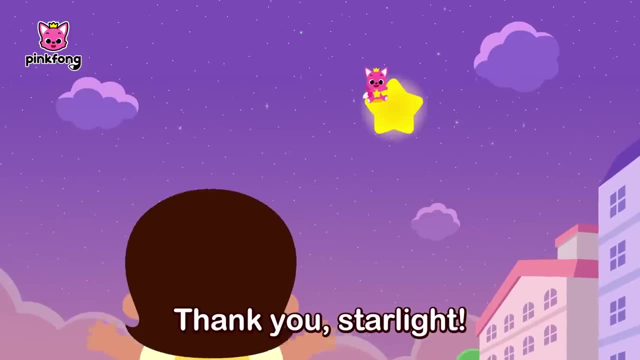 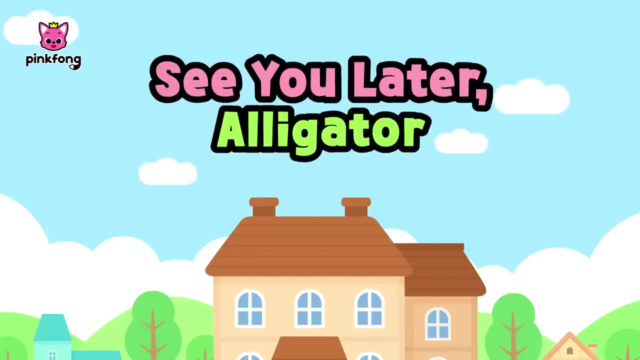 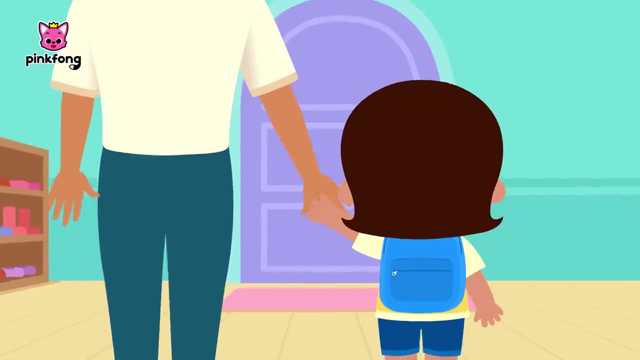 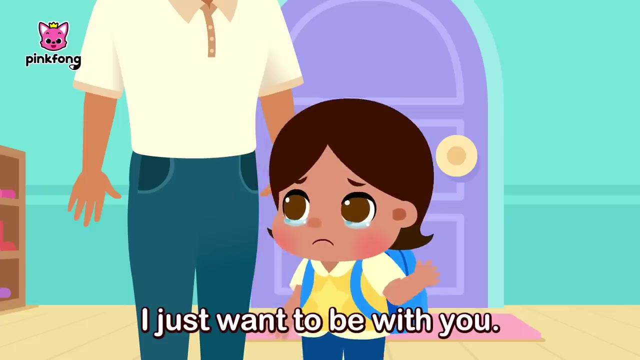 Hey, it was a fun day today, Thank you, thank you, thank you. See you tomorrow. See you, Thank you, Starlight. Good morning, sweetie. It's time to go to school. No, no, don't leave me, Daddy, I just want to be with you. 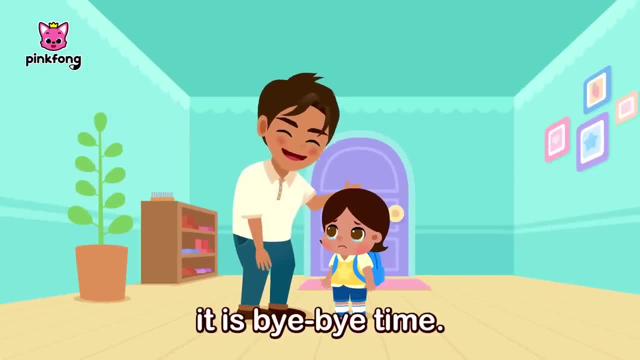 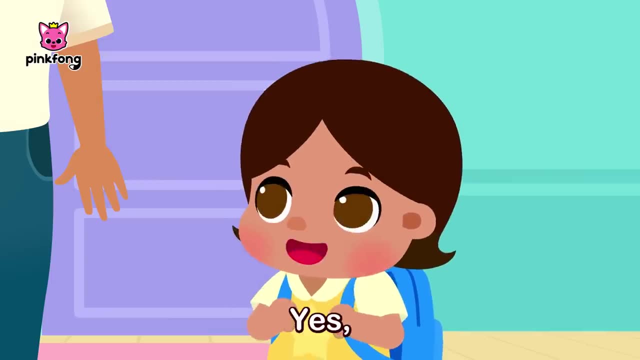 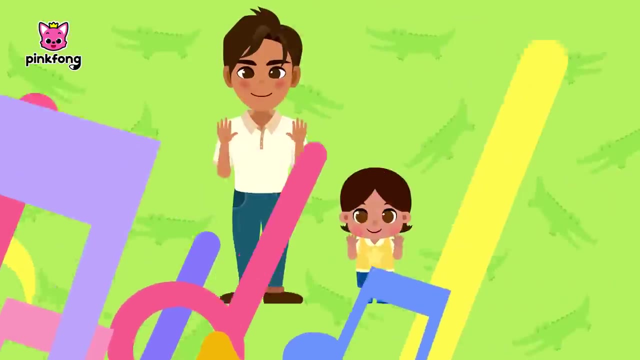 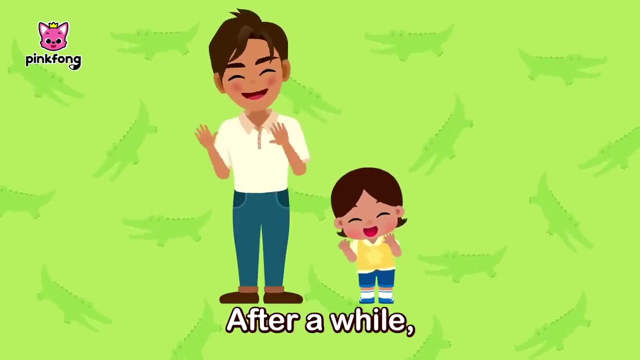 Sweet baby, it's time to go to school. It is bye-bye time. Do you remember the alligator song? Yes, I do remember. Let's sing it together. See you later. alligator, After a while. crocodile, Then give a hug and a kiss. 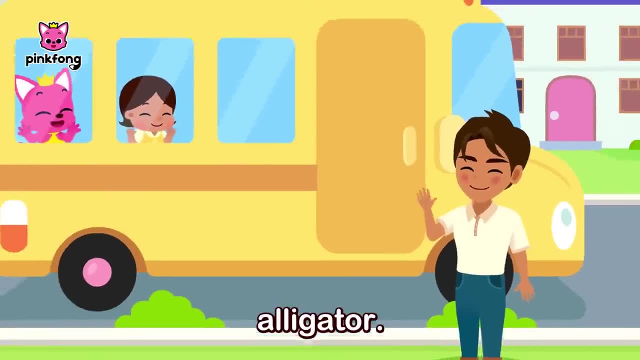 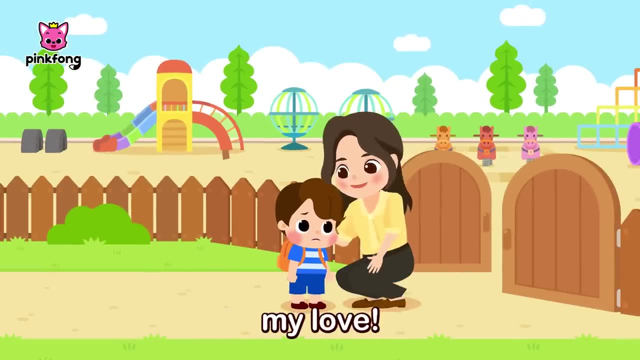 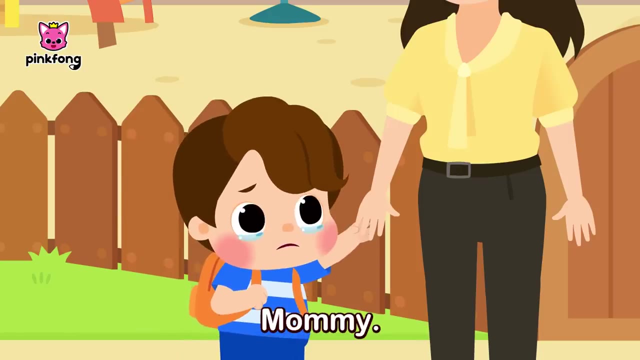 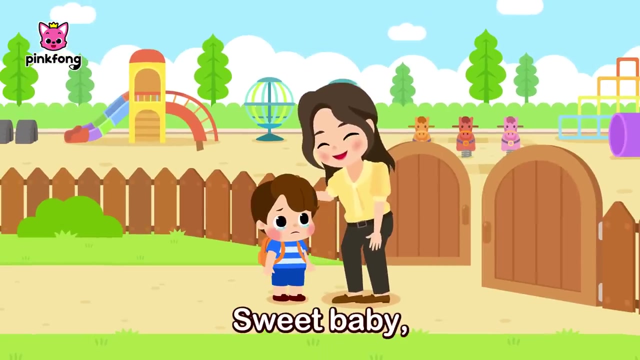 Bye-bye. See you later, alligator Bye-bye. have a great day, my love. No, no, don't leave me, Mommy, I just want to be with you. Sweet baby, it is bye-bye time. Do you remember the alligator song? 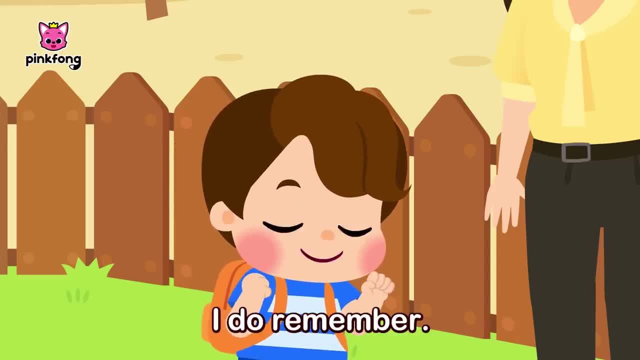 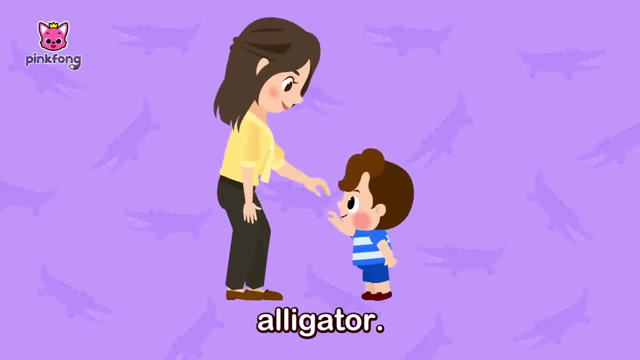 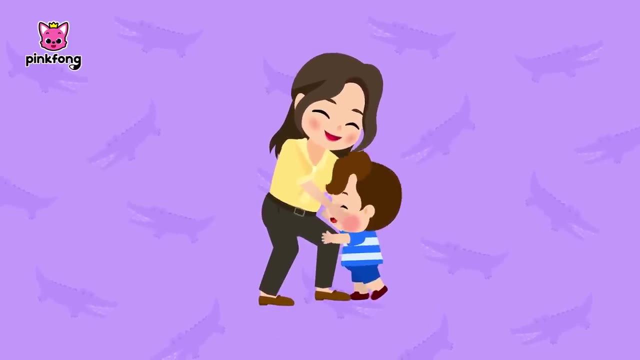 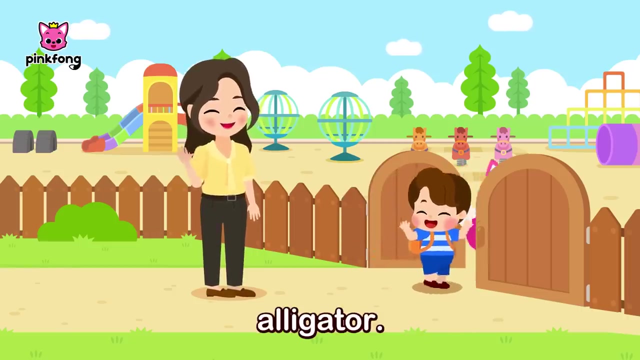 Yes, I do remember. Let's sing it together. See you later, alligator. After a while. crocodile. Then give a hug and a kiss: Bye-bye, see you later, alligator. See you later, alligator, After a while, crocodile. 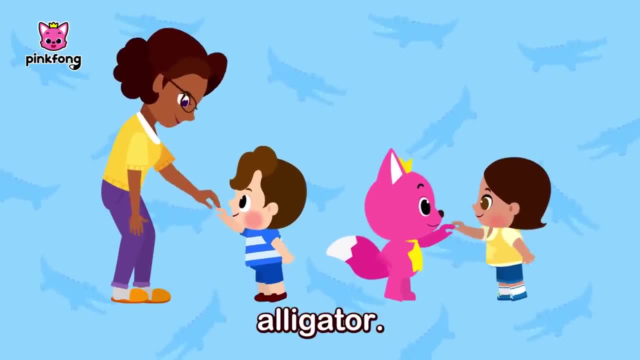 Then give a hug and a kiss Bye-bye. see you later, alligator. See you later, alligator, After a while. crocodile: Then give a hug and a kiss Bye-bye. see you later, alligator, After a while. crocodile. 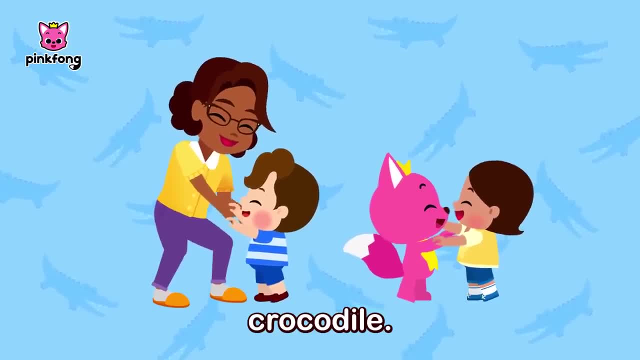 Then give a hug and a kiss Bye-bye. see you later. alligator- After a while. alligator, Then give a hug and a kiss Bye-bye. see you later. alligator- After a while. alligator- After a while. alligator. 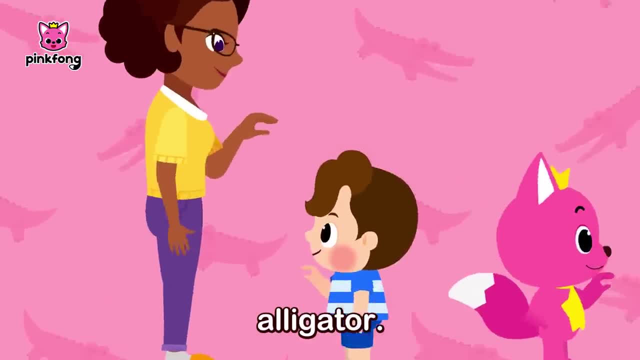 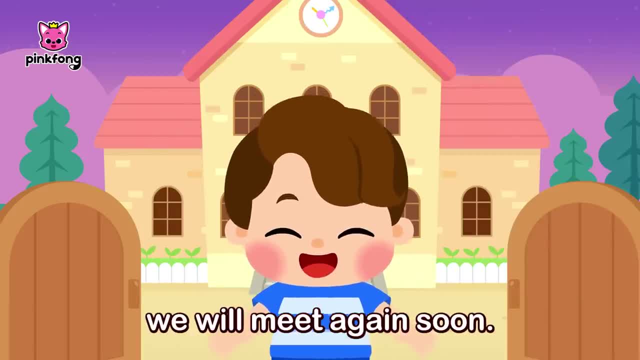 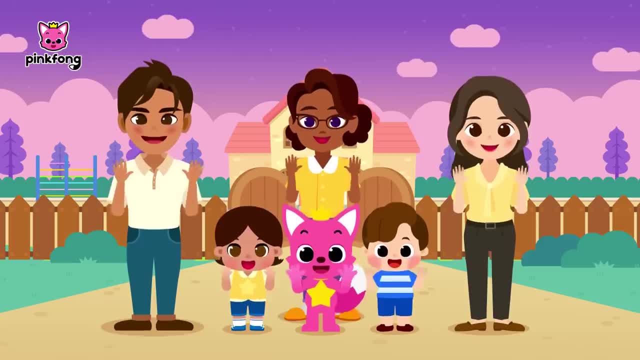 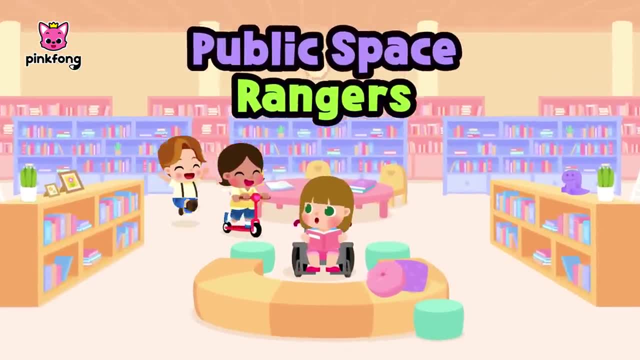 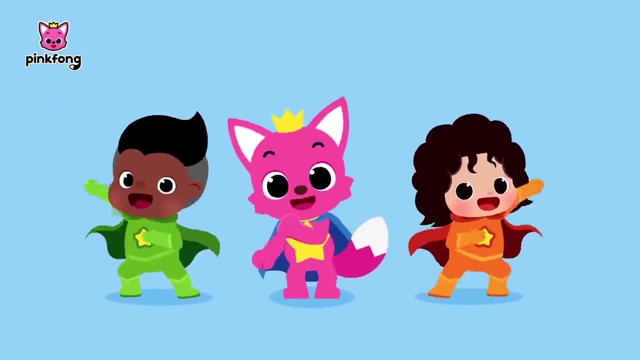 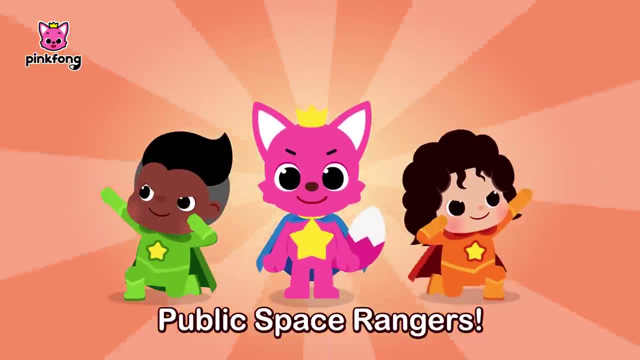 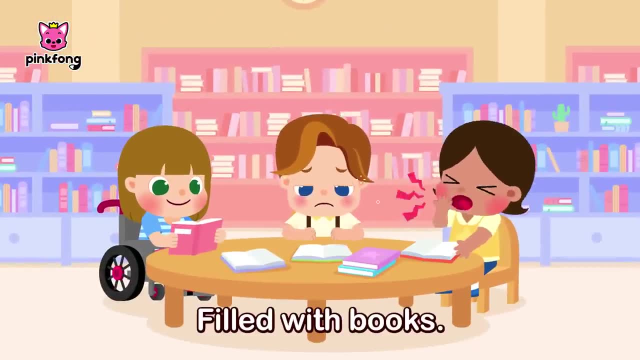 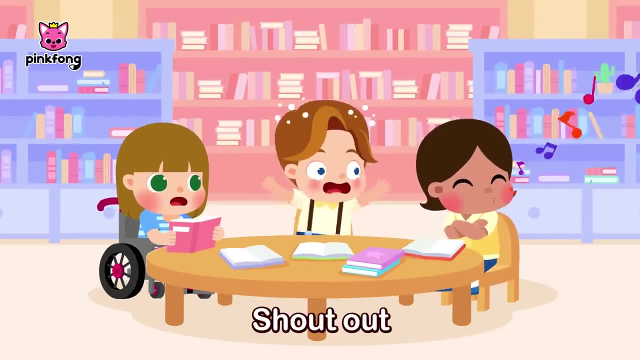 Whoa, whoa, whoa. Public Space Rangers At the library. Books, books filled with books. Everyone is so quiet. Let's play tag, tag, tag tag. Shout out to your friends, Stop, Listen to the Public Space Rangers. 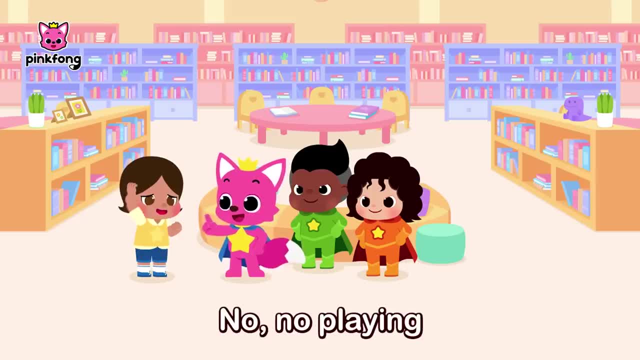 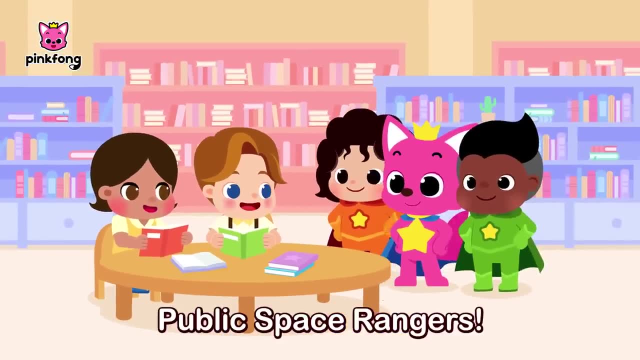 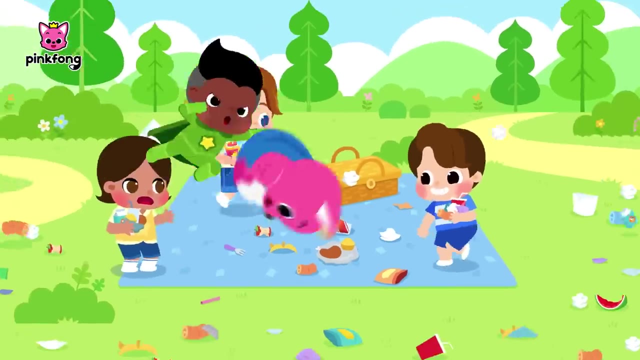 No, no shouting in a public space. No, no playing in the library. Let's keep our manners. Now we're all Public Space Rangers. Hey, let's play catch with this garbage. Not in the public space. Public Space Rangers. 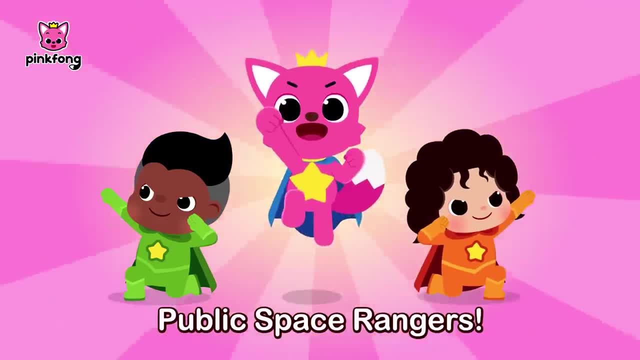 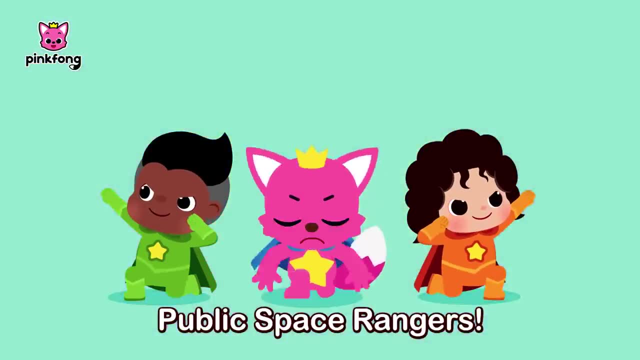 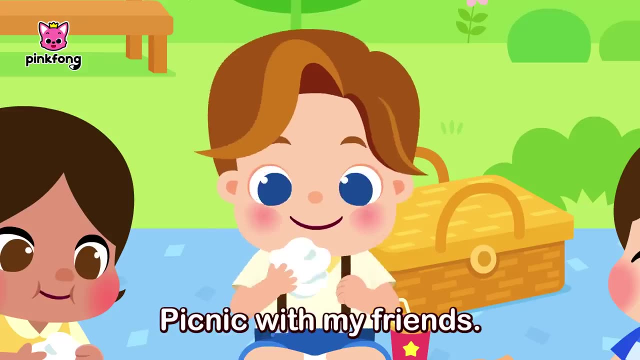 Whoa whoa whoa Public Space Rangers. Public Space Rangers. Whoa whoa whoa Public Space Rangers At the park. Sunny, sunny. it's a sunny day, Picnic with my friends, Throw trash and play games. 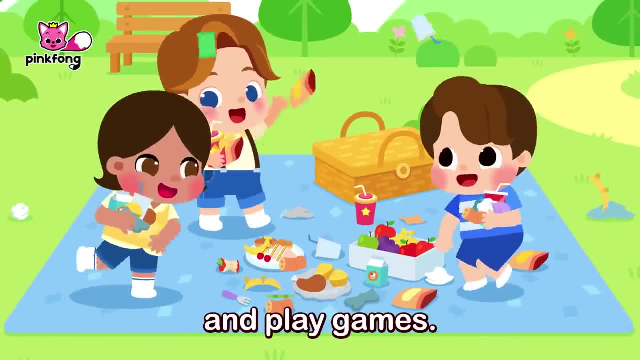 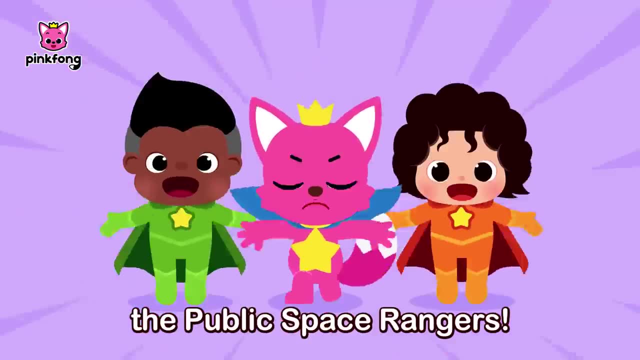 Litter and make a mess. Stop Listen to the Public Space Rangers. No, no littering in a public space. No, no making a mess in the park. Let's keep our manners. Stop Listen to the Public Space Rangers. 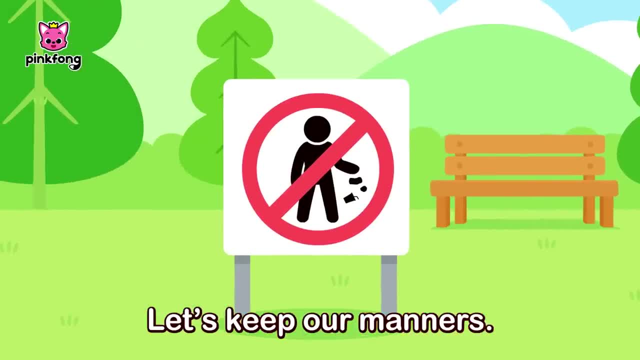 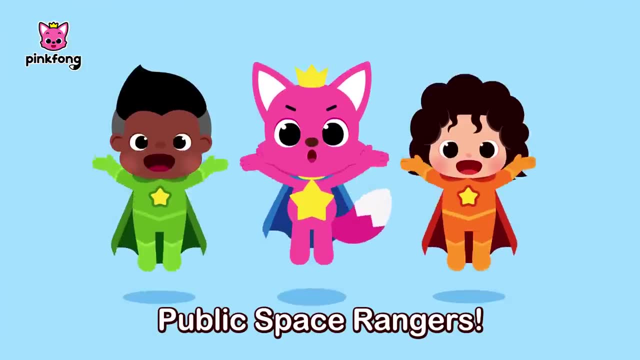 No, no littering in a public space. No, no, making a mess in the park. Let's keep our manners. Now we're all Public Space Rangers. Public Space Rangers. Whoa, whoa, whoa. Public Space Rangers. 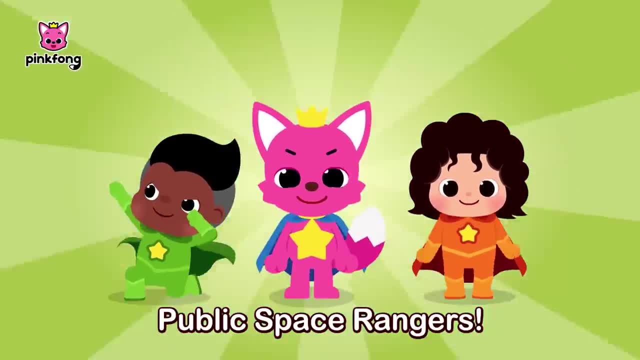 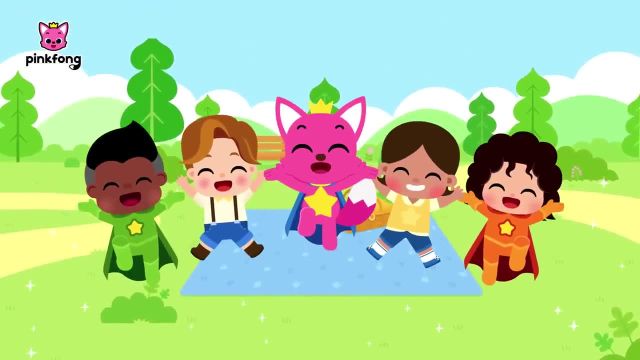 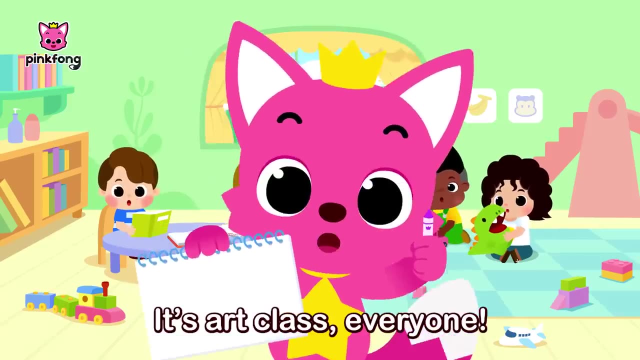 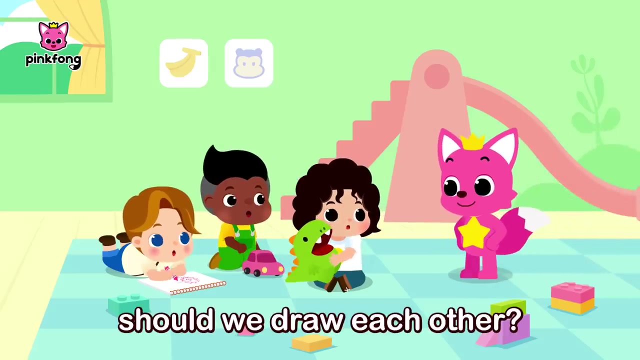 Public Space Rangers. Whoa, whoa, whoa. Public Space Rangers. We are all Public Space Rangers. It's art class. everyone, Let's draw. Hey, since we're best friends, should we draw each other? Totally? Let's go grab some crayons. 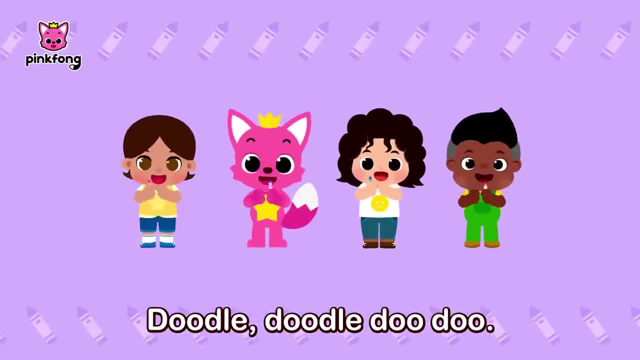 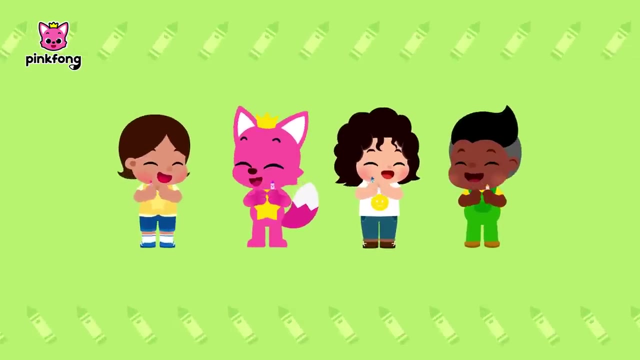 Yay. Doodle doodle doo doo. doodle doodle doo doo. Time to draw, draw, Draw. Doodle doodle doo doo. doodle doodle doo doo. Time to draw, draw, Draw, Draw, draw. my friends, let's draw. 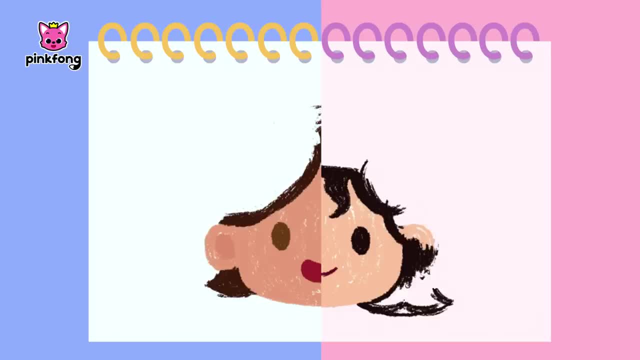 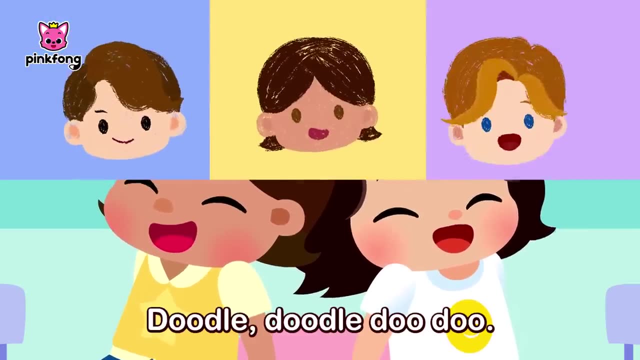 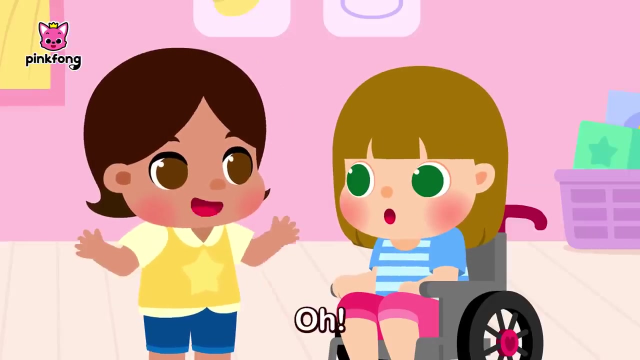 Take a close look at my friends. I have curly hair and you have straight hair. Everyone's special in their own way. Doodle, doodle, doo, doo, doodle, doodle, doo doo. Time to draw, draw. Oh, we don't have the same eye color. 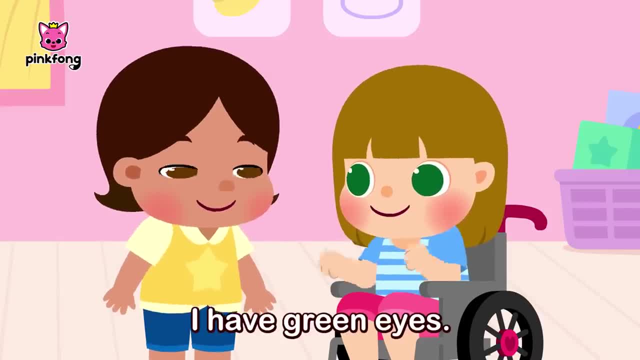 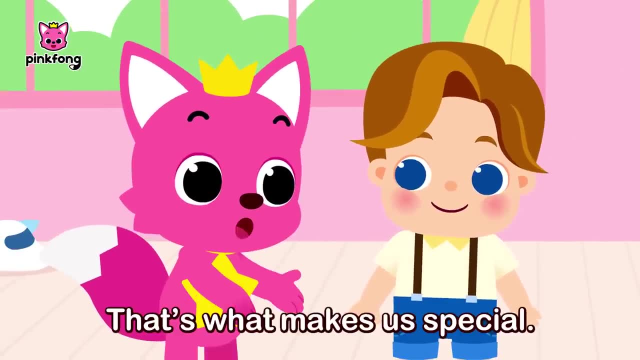 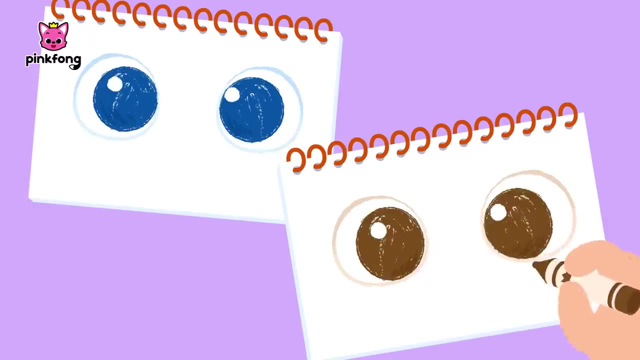 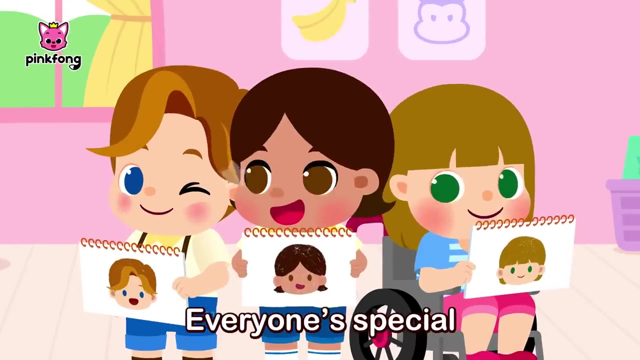 You're right, I have green eyes, I have brown eyes, Mine are blue. Everyone has different eye colors. That's what makes us special. Like a rainbow. Different eye colors like a rainbow, Different nose shapes, like pebbles. I am different, I am special, Everyone's special in their own way. 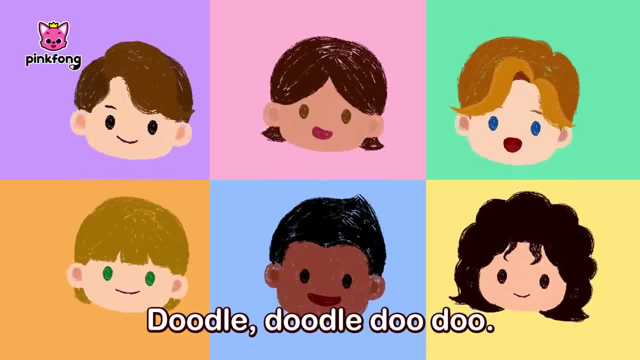 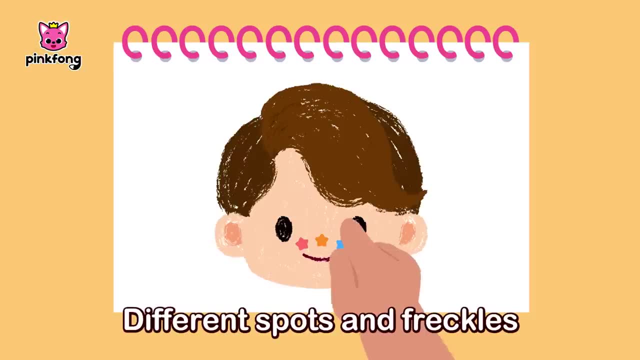 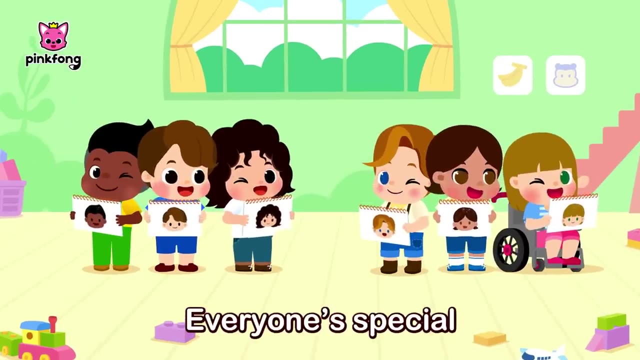 Doodle, doodle, doo doo, doodle, doodle, doo, doo. Time to draw. draw Different skin colors like a palette, Different spots and freckles, like the stars. I am different. I am special, Everyone's special in their own way. We are special. la, la, la la. 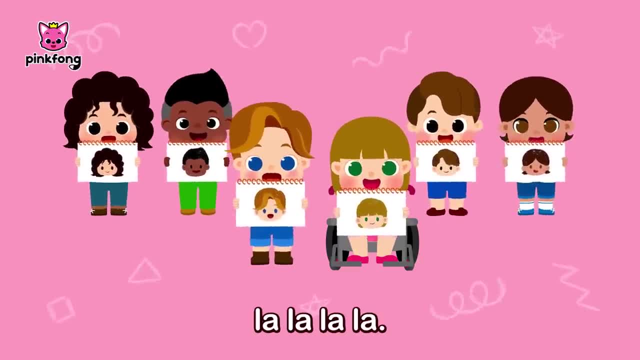 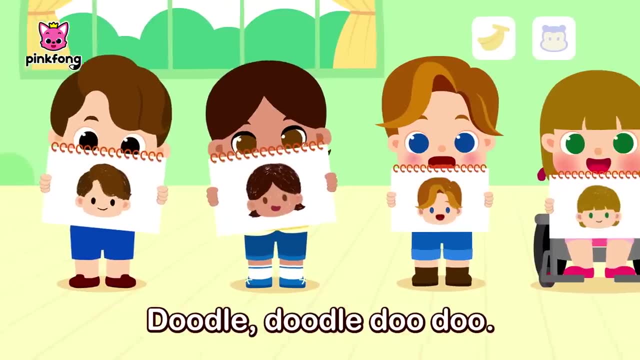 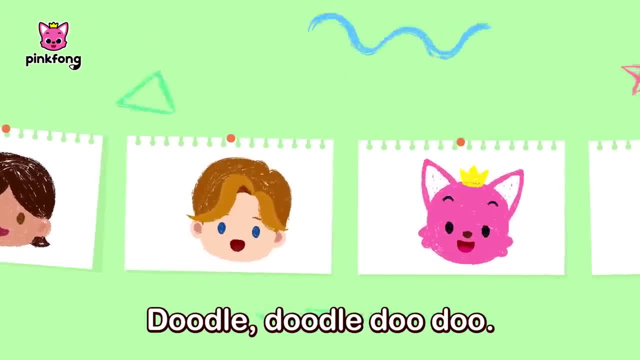 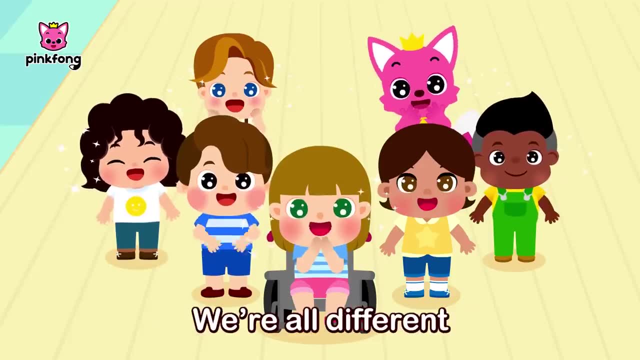 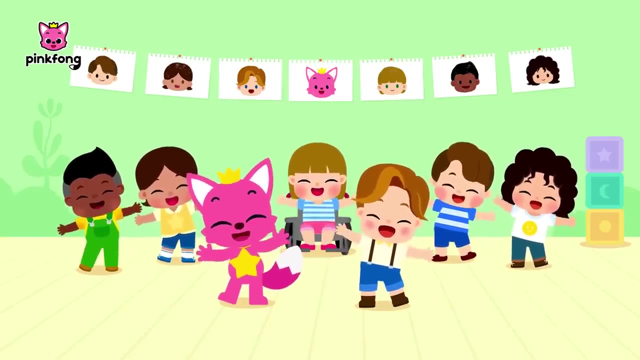 Draw: Doodle, doodle, doo doo, doodle, doodle, doo doo. Time to draw, draw, Draw. Wow, look at all our friends. We're all different and beautiful, Which makes us all special. Ha ha, ha, ha, ha, ha ha. 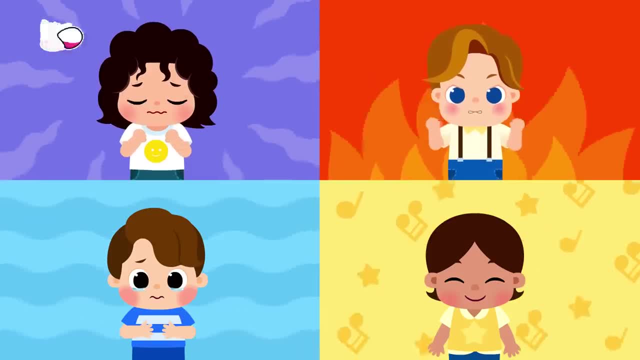 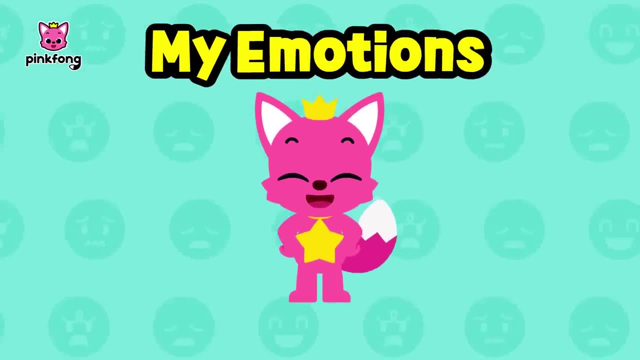 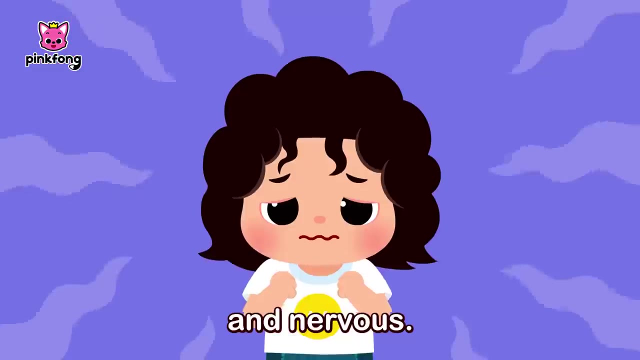 I'm so nervous, I'm so angry, I'm so sad, I'm so happy, I'm so happy. Hey, let's share our feelings. My, oh my emotions. I clearly have. I said: I'm free and nervous. That's all me. When are you nervous? 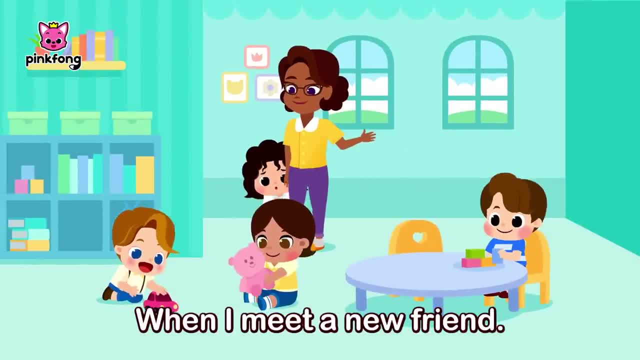 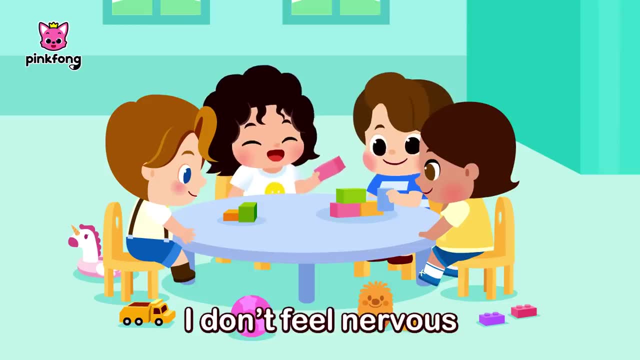 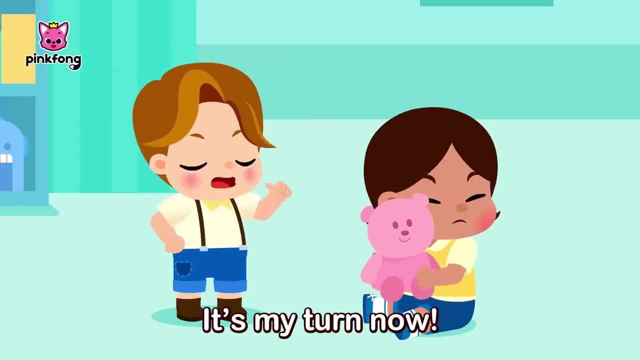 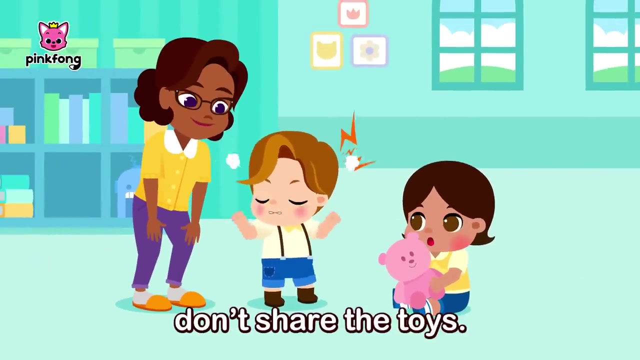 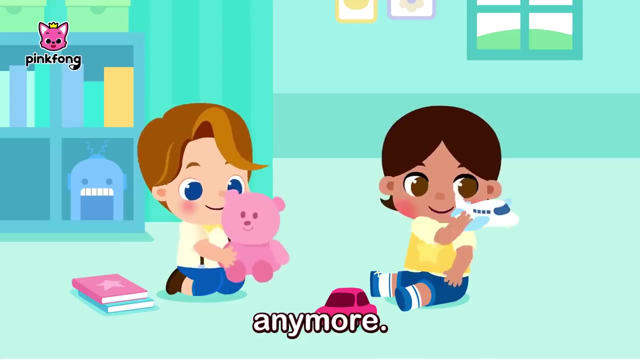 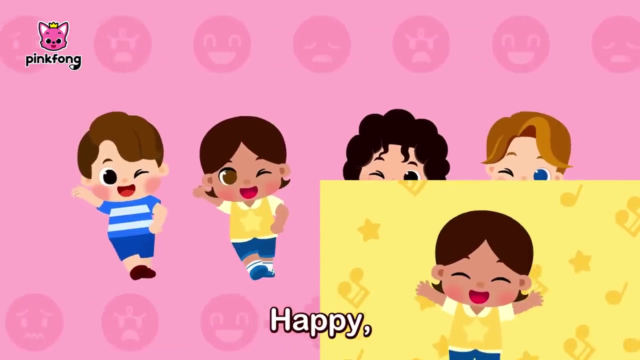 I get nervous. I get nervous When I meet a new friend, But after we say hi and play together, I don't feel nervous anymore. I feel Sophia, I get nervous. I feel richtige. I say hi again. I feel nice. I feel B. I feel really good. Tell me, when are you sad? 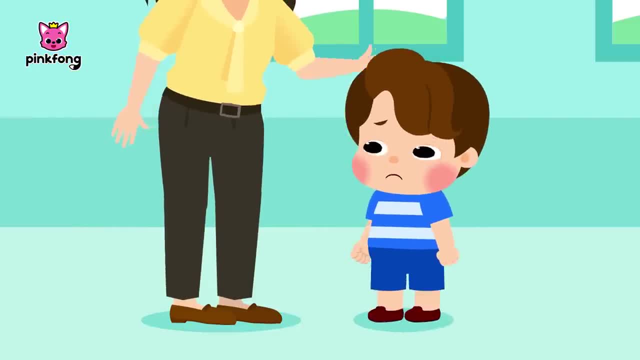 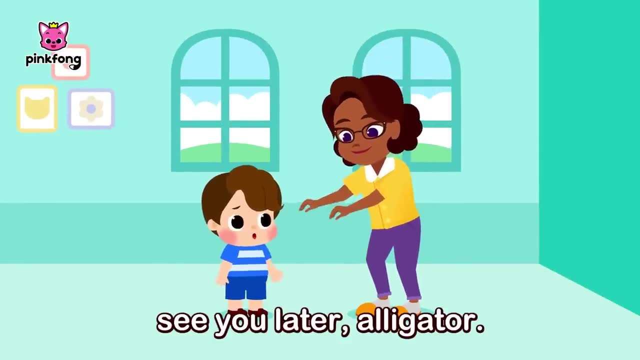 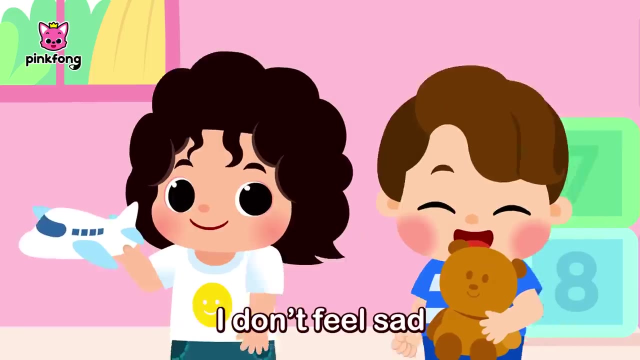 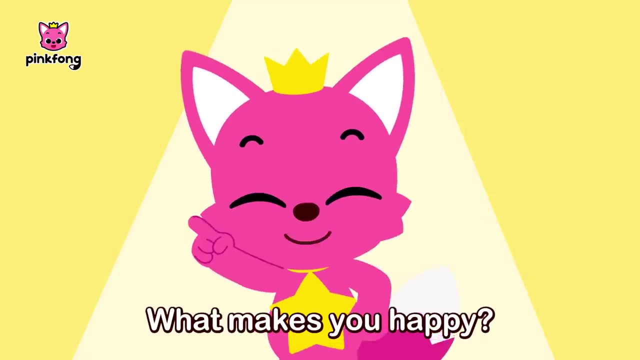 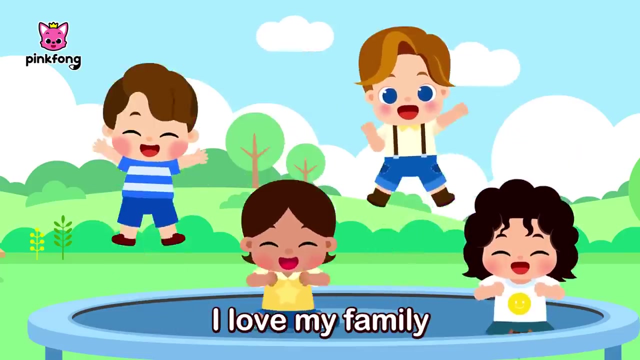 I get sad. I get sad When I say goodbye to mom and dad. It's okay, see you later, alligator. Hey, come and play. Okay, I don't feel sad anymore. What makes you happy? I am happy When I spend time with my loved ones. 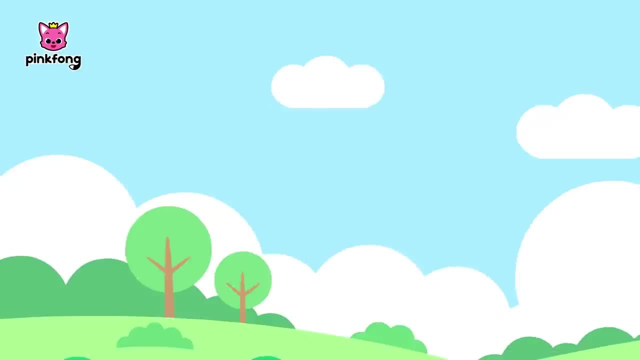 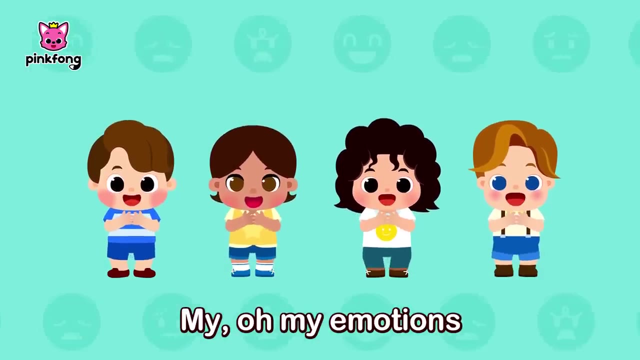 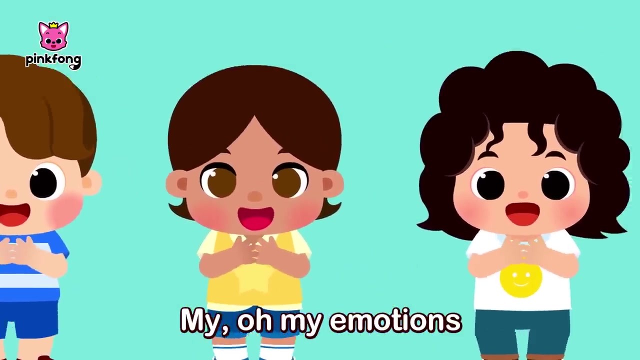 I love my family and friends so much. I am happy, happy, My, oh, my emotions. I feel like I'm sad, angry and nervous. My, oh, my emotions. I feel like I'm sad, angry and nervous. That's all me. We are happy. 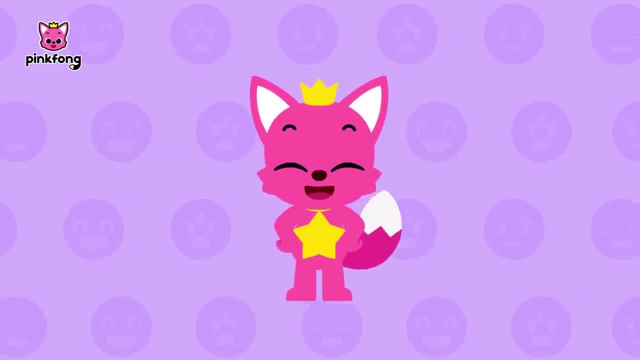 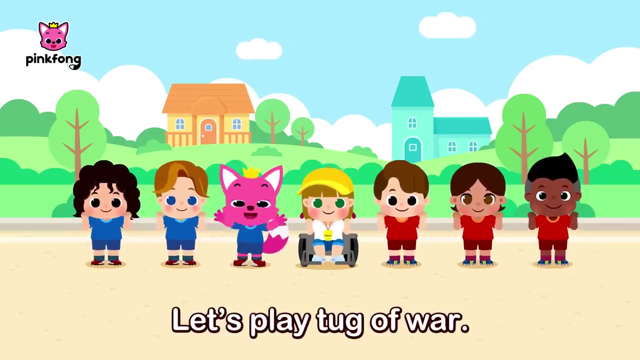 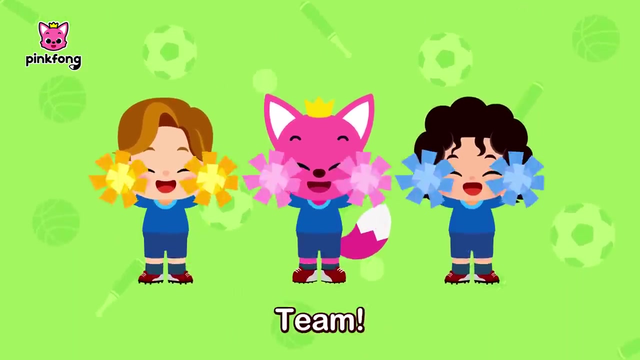 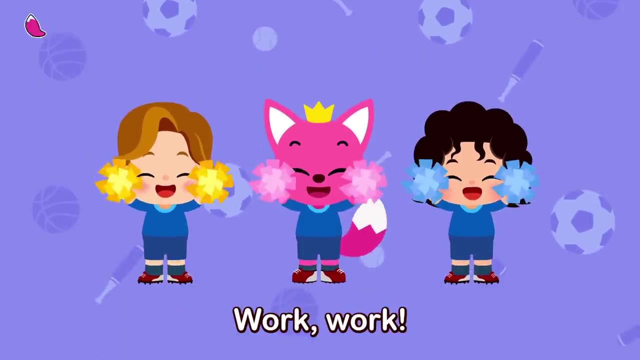 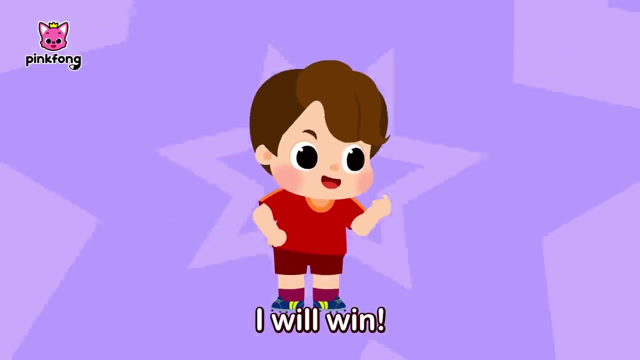 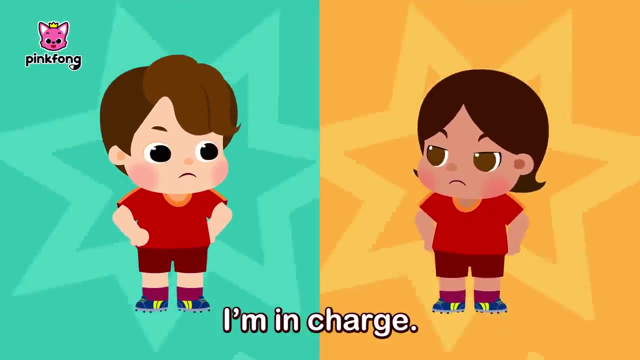 We love you, no matter how you feel. Tug of war. tug of war, I will win. No, I will win. Get out of my way, Out out everyone. It's me. me, I'm in charge. No, no, I'm in charge. 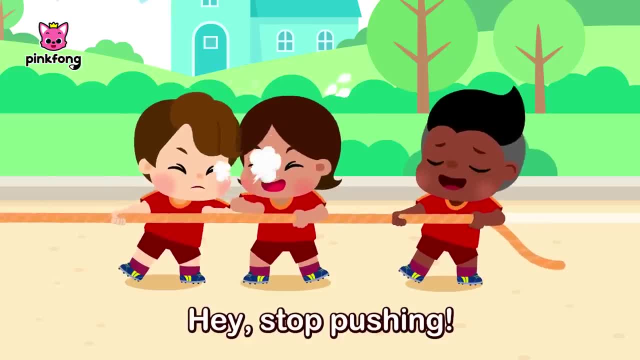 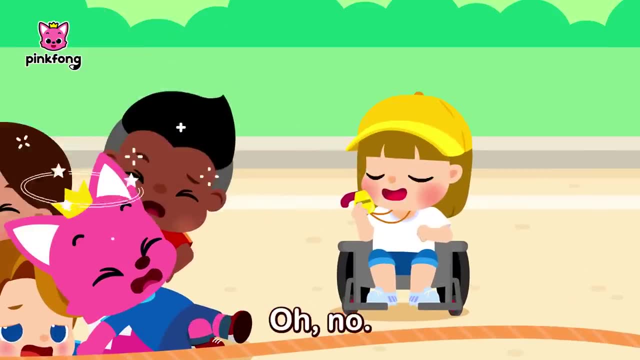 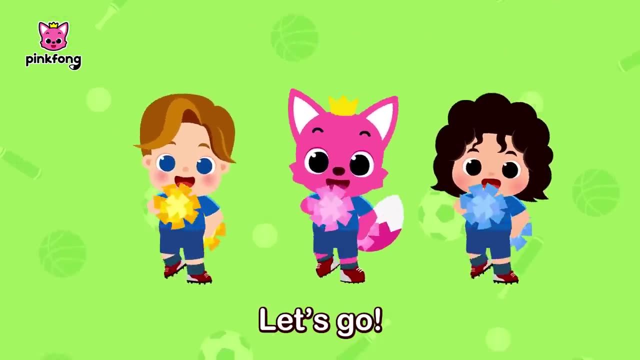 I don't need anyone. Hmph, hey, stop pushing, Get out of my way. Ouch, you stepped on my foot, Arrgh. Oh no, they're not working as a team. Let's show them what teamwork is all about. Let's go. let's go. 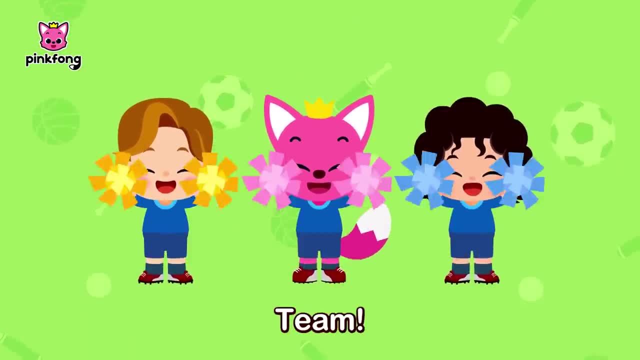 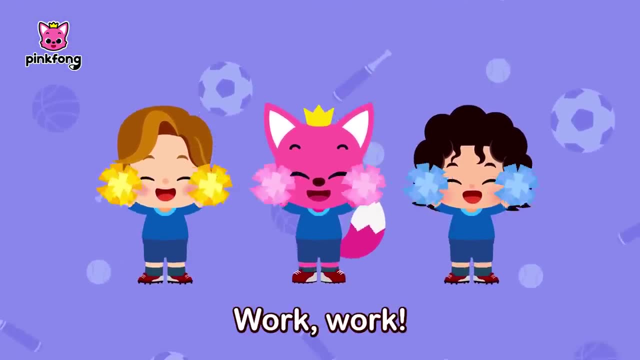 We can do it all together: team Work, work, Team Work, work. Let's go, let's go. We can do it all together. team Work, work, Team Work, work. Kick the ball, pass the ball. We will win, win, win. We can do it all together. here we go, everyone. 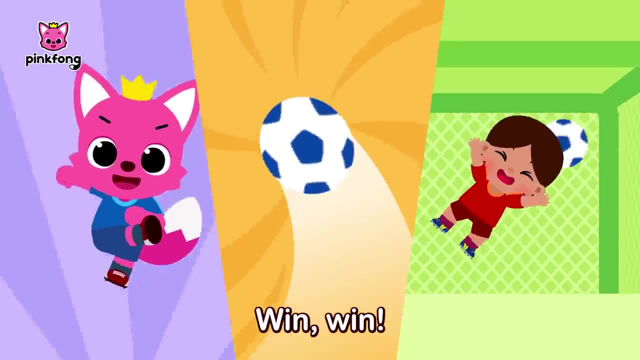 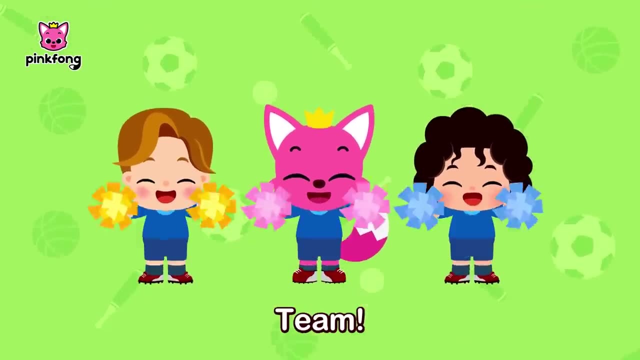 You and me, us together, We will win, win, win. Let's show our teamwork. Let's go, let's go. We can do it all together. team Work, work, Team Work, work. Let's go, let's go. We can do it all together. team. 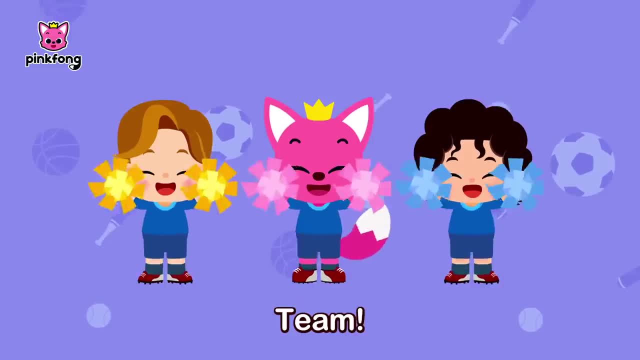 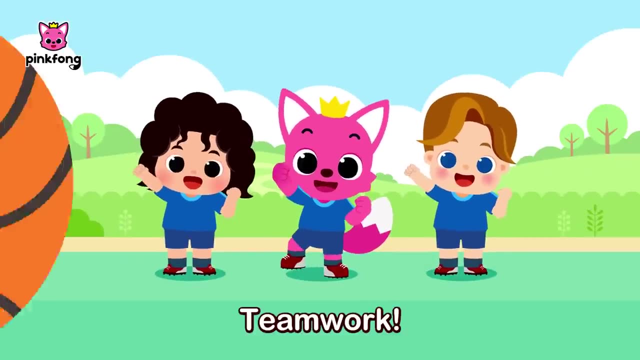 Work, work, Team Work, work, Team Work, work. Ugh, how come we never win? We know what you need: Teamwork. Thump the ball, shoot the ball. We will win, win, win. We can do it all together. here we go everyone. 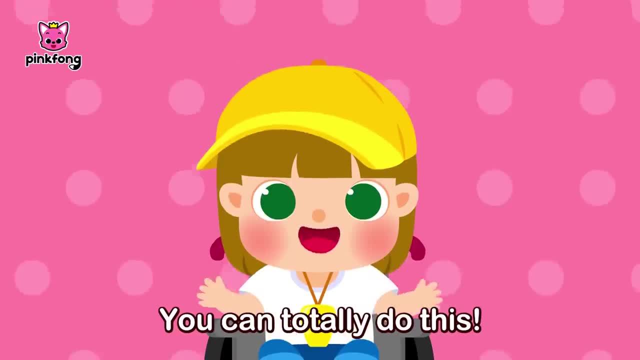 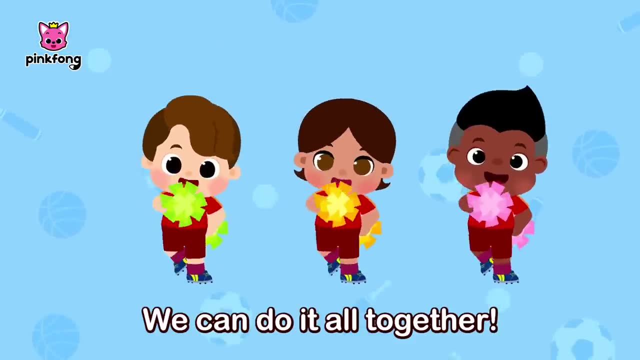 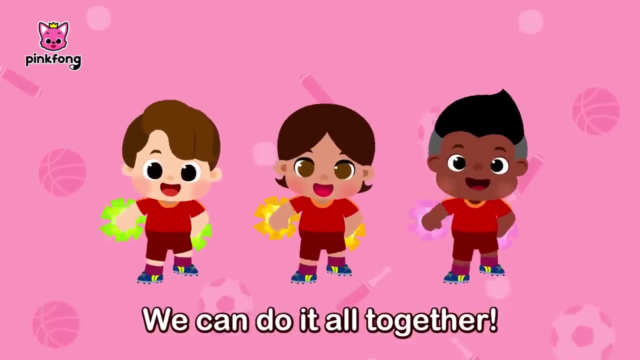 You and me, us together, we can do this. You can totally do this. Now let's show our teamwork. Yay, Let's go, let's go. We can do it all together. team, Team Work, Work, Team Work, Work. Let's go, Let's go, We can do it all together. 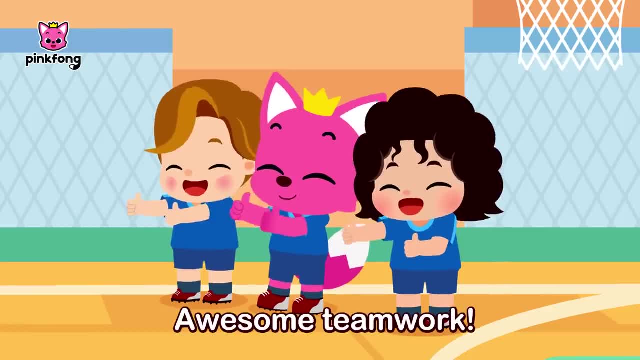 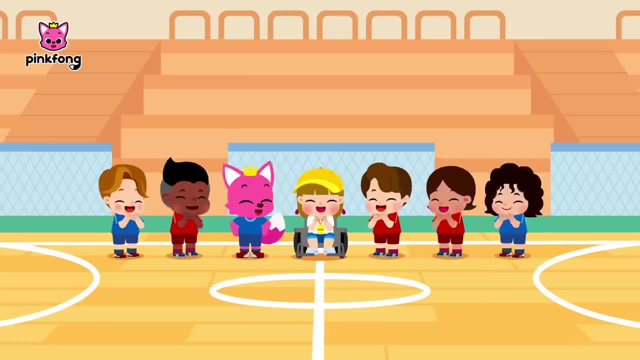 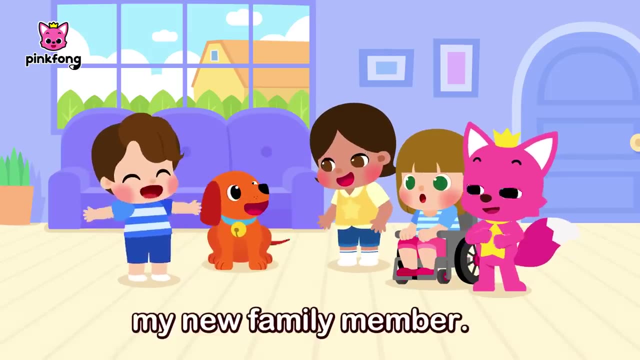 Team Work, Work, Team Work, Work, Awesome teamwork. You are winners today. Working as a team is great. Hey Say hi to my new family member. He's my little brother. Aww, Your puppy is so cute. 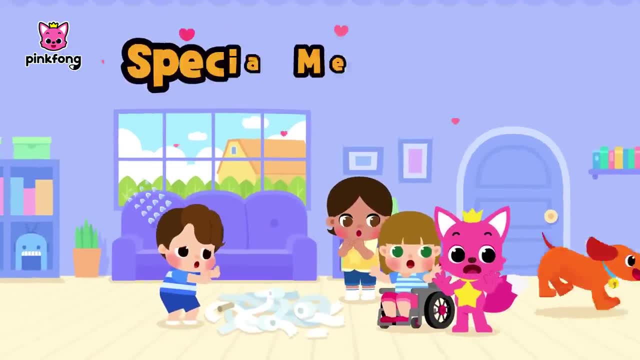 Oh no, Look at all the mess he made. Oh no, Look at all the mess he made. Uh-oh, Will he be in trouble? My little brother doo-doo-doo-doo-doo. My little sister doo-doo-doo-doo-doo. 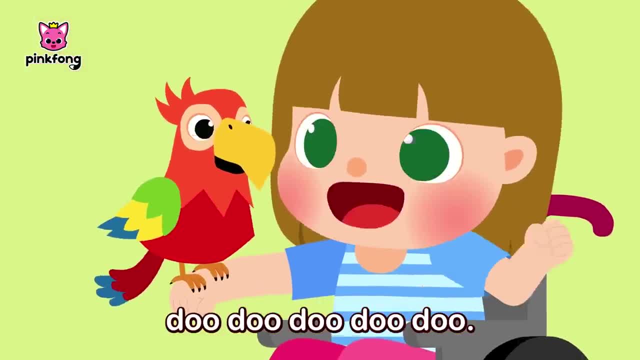 My little sister doo-doo-doo-doo-doo, My best friend doo-doo-doo-doo-doo, My best friend doo-doo-doo-doo-doo. I love you, doo-doo-doo. 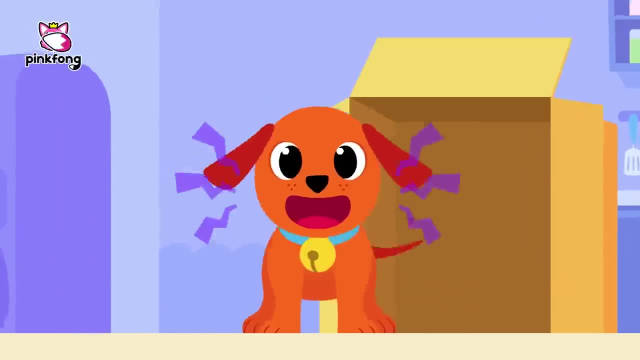 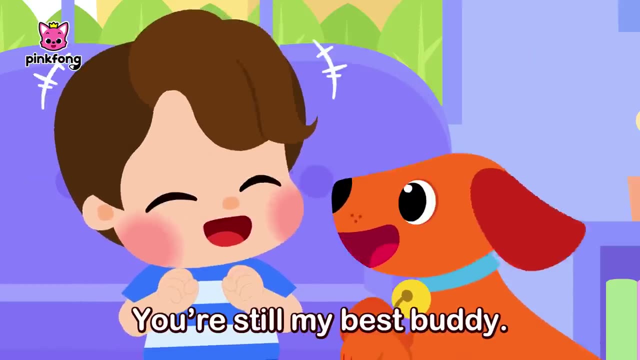 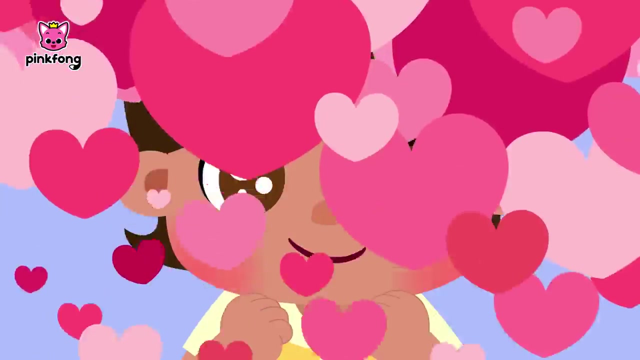 My little brother is a happy, goopy puppy. I throw, catch and pull A game of tug-of-war, But no, no worries, You're still my best buddy, My puppy, my brother, You two are so cute, I have a kitty. 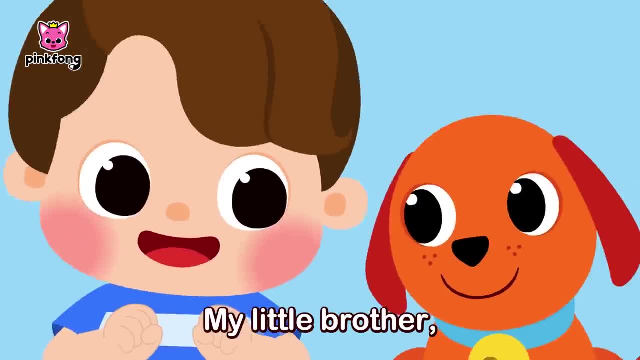 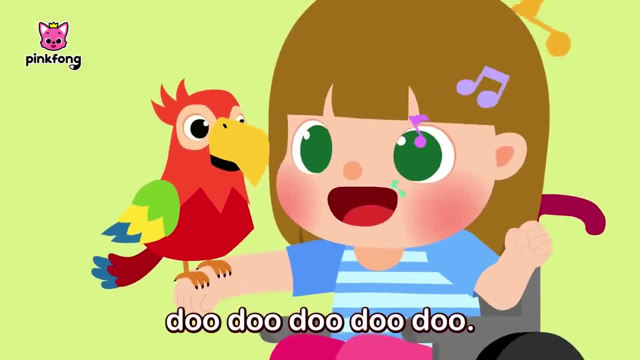 She's my little sister, My little brother doo doo doo doo doo. My little sister, doo doo doo doo doo, My best friend. doo doo doo doo doo. 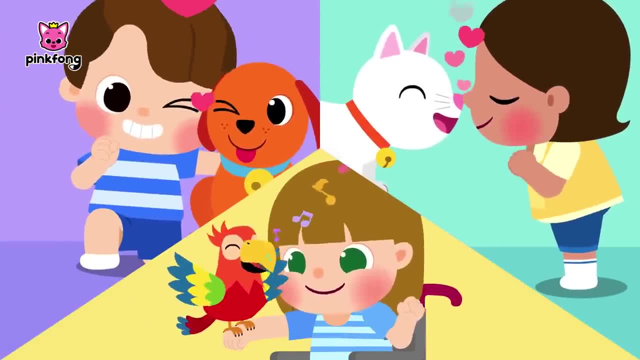 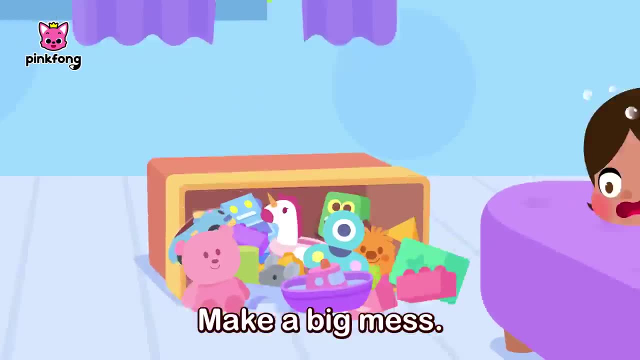 I love you. doo, doo doo. My little sister is a happy, fluffy kitty. We run, jump and climb, Make a big mess. Oh no, Get into trouble when we're having fun. As long as we have each other, we'll be OK. 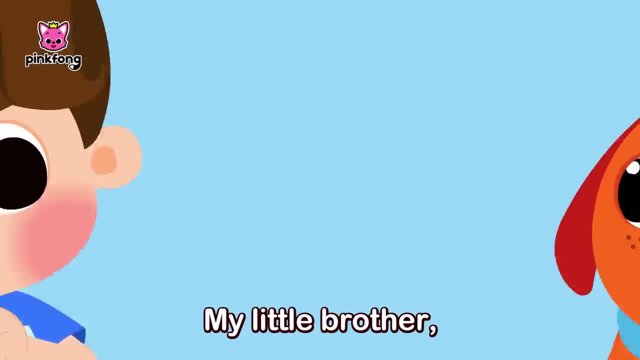 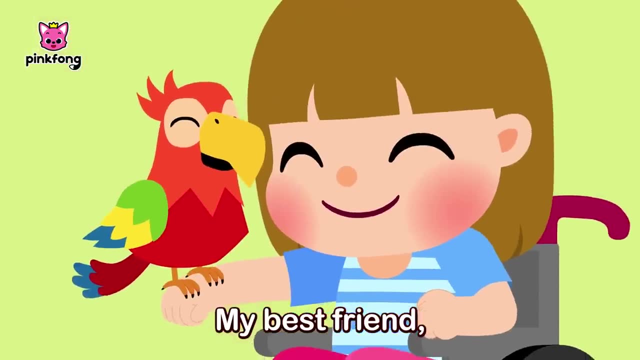 My kitty, my sister, My little brother doo doo doo doo doo. My little sister doo doo doo, doo doo, My best friend, doo doo doo, doo doo. 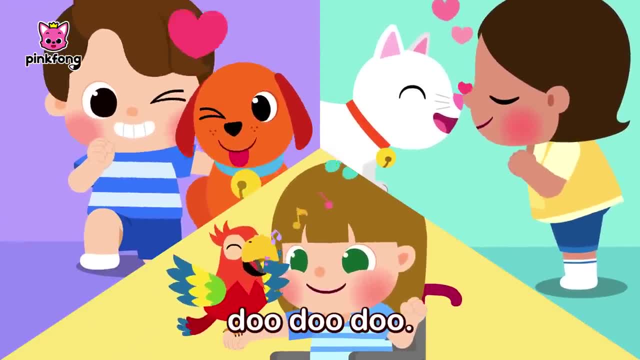 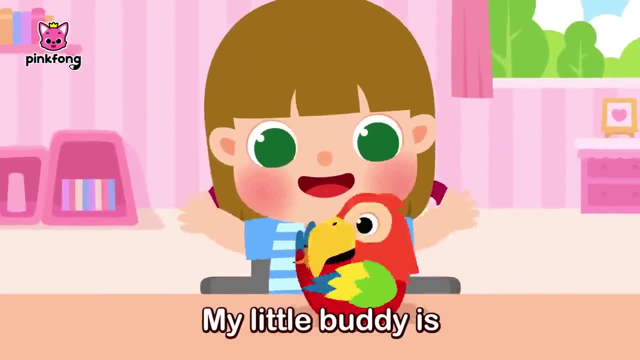 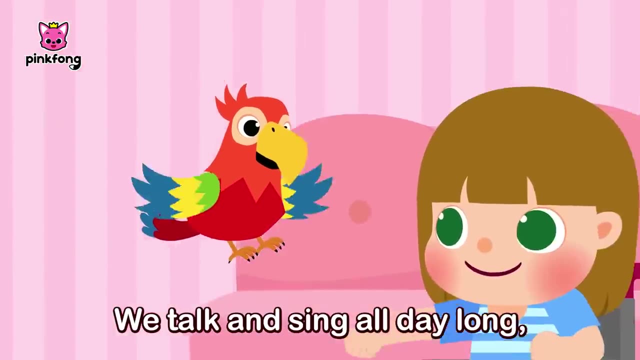 I love you. doo, doo doo. Do you have a special member? Your family, My little buddy is a happy, smarty birdie. We talk, chat and chat, Hello, Hello. We talk and sing all day long. 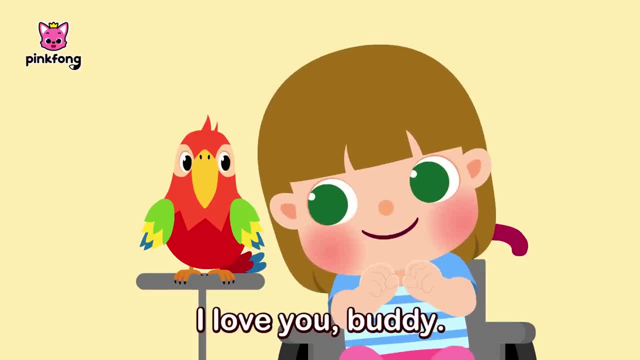 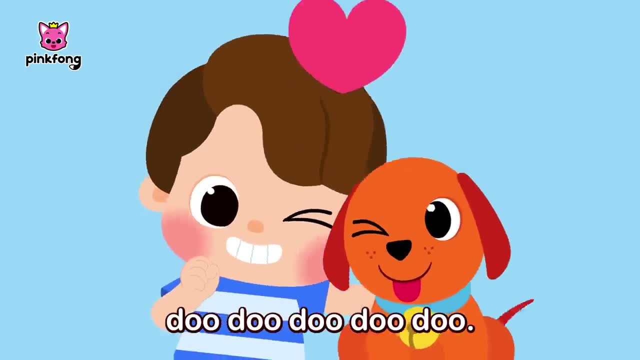 La, la, la, la la. I love you, buddy. I love you too, My birdie, my buddy, My little brother doo doo, doo, doo doo. My little sister doo doo, doo, doo doo.